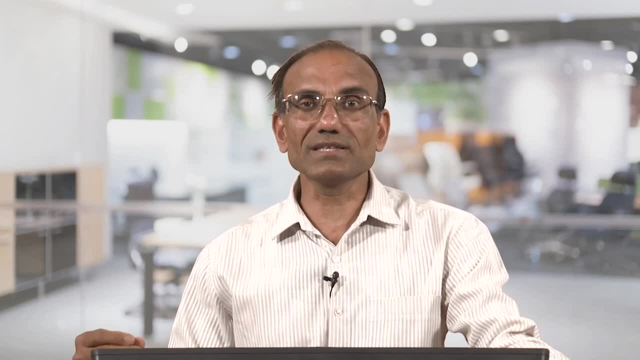 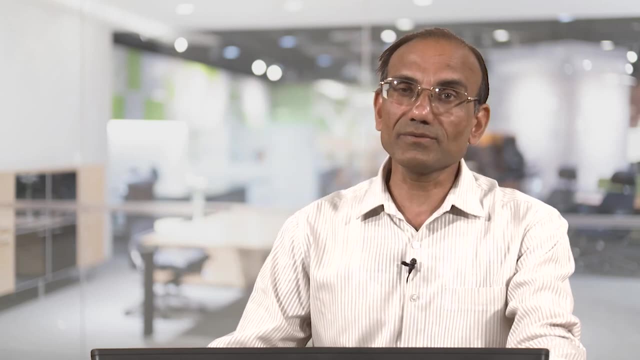 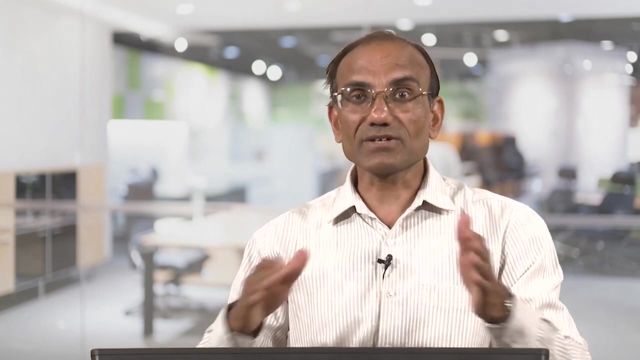 of these vibrations is so small, so thin that we are not able to even feel that. And these vibrations, like you know, the amplitude may vary, which may be in nanometers to in the meters. Similarly, when we talk about its wavelength, it may be also quite varying, So frequency. 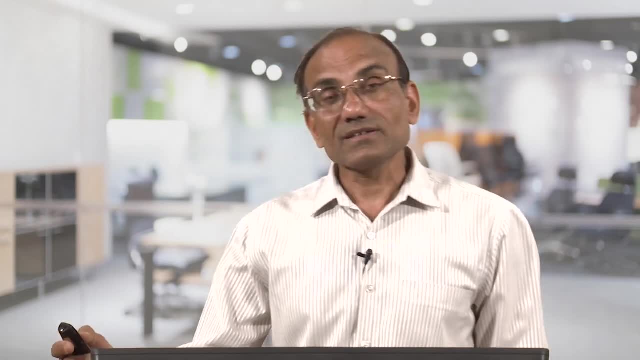 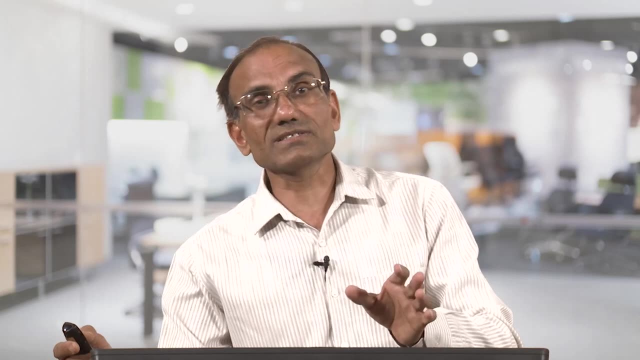 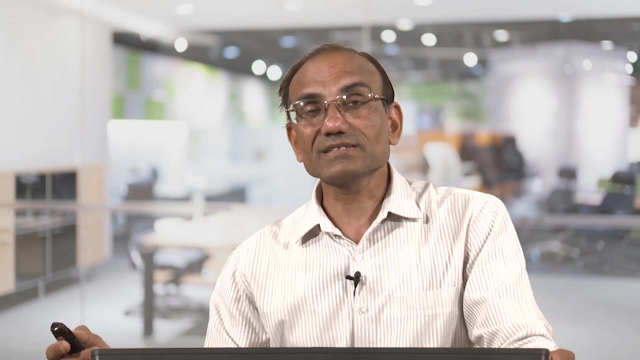 content will also much varying. So now, as a for seismologist, the small vibration is also important for the research and other purpose. but as for engineers, particularly like geotechnical earthquake engineering discipline and other things, it is a strong ground motion. 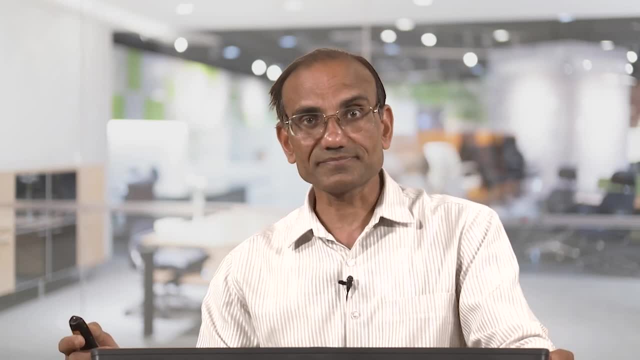 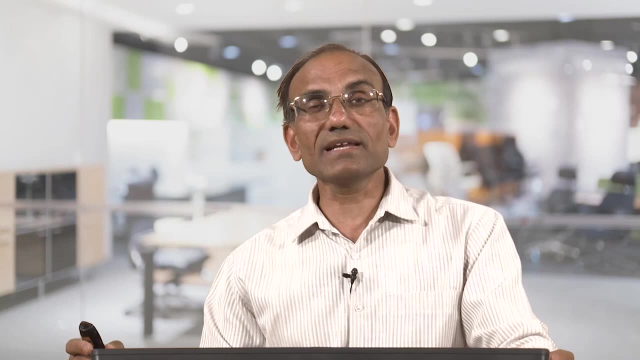 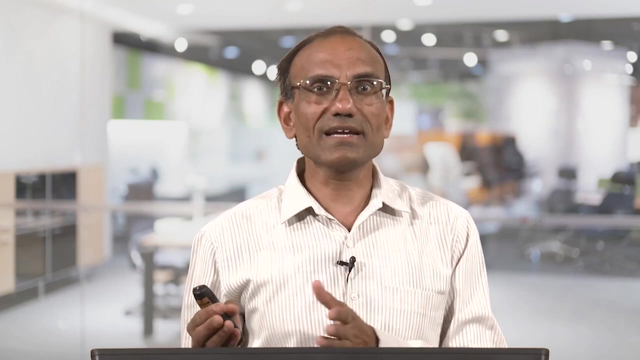 which is most important, and today we are going to talk about that. Now, coming to this, as I just mentioned, the earthquake engineers are interested primarily in strong ground motion, That is, the motion which have sufficient strength to affect people and their environment. So if suppose some vibrations are coming with which do not have 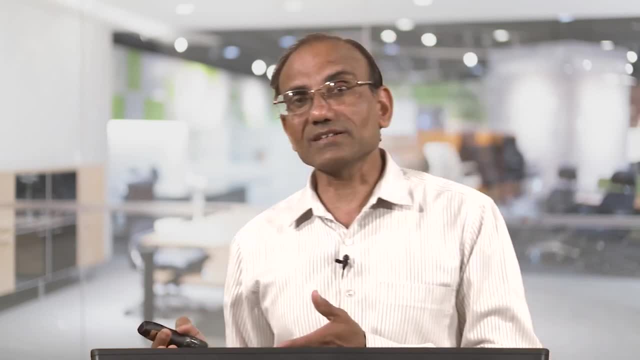 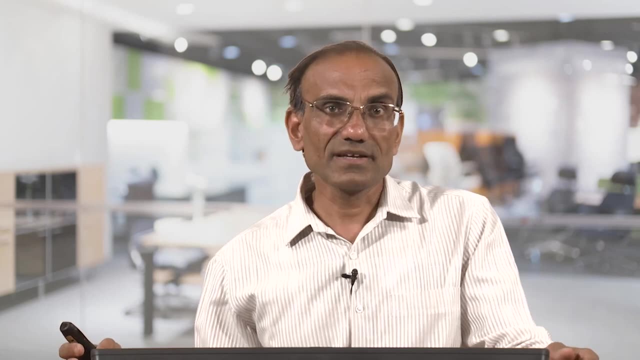 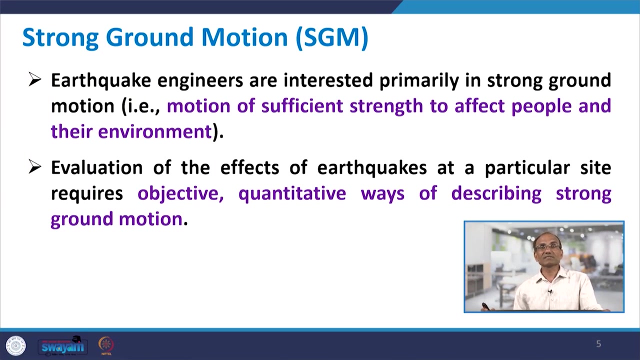 any effect on livelihood or let us say on like, on environment, then it is not so important for engineers To evaluate the effects of earthquakes at a particular site. it requires quantitative ways of describing strong ground motion. We need to quantify that in different parameters. 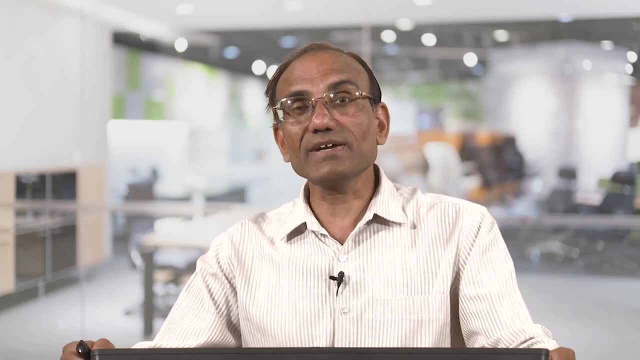 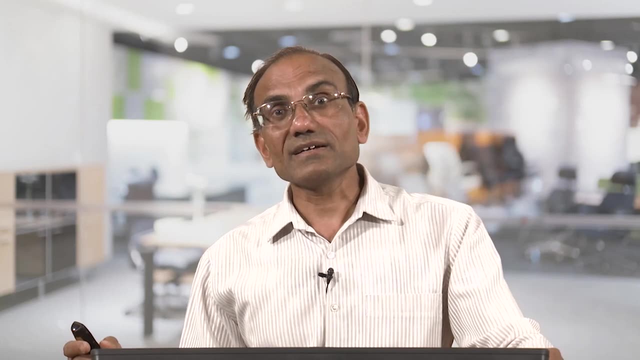 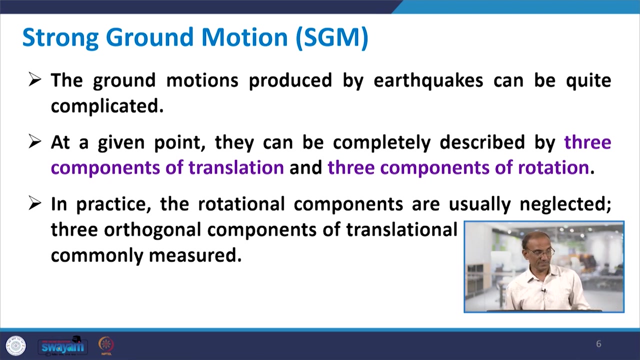 so we? what are the parameters which quantify this strong ground motion we are going to talk today? Continue with this. the ground motions which is produced by earthquakes. they are mostly quite complicated. At a given point they can be completely described by what we say. three component of translation. 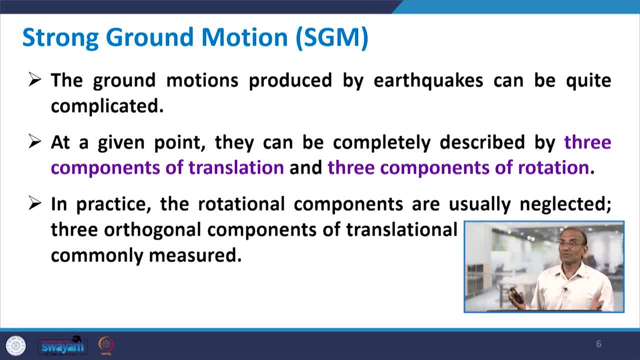 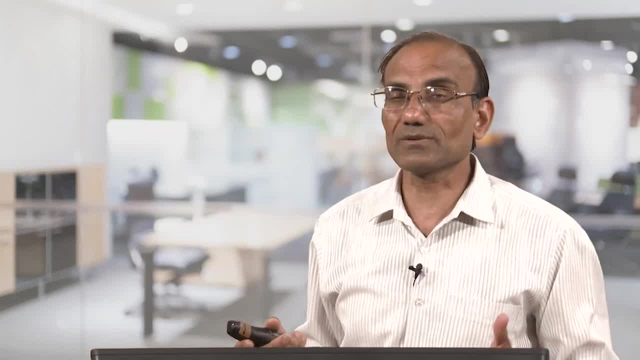 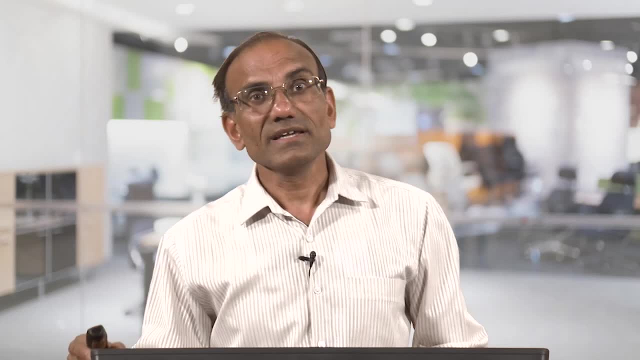 and three components of rotation. In 3D space you have three components of translation like this and the rotation also. So you have x y z, normally the coordinates. So in the x y z you may have displacements and then you may have rotations also. 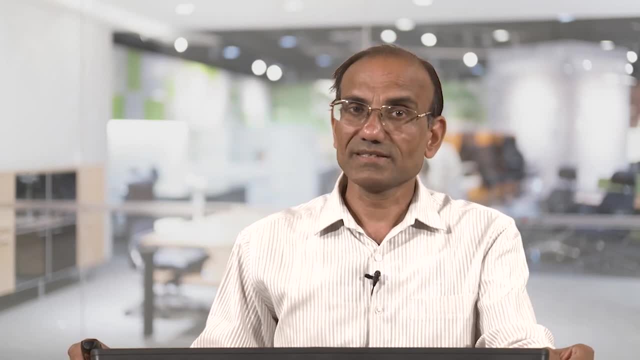 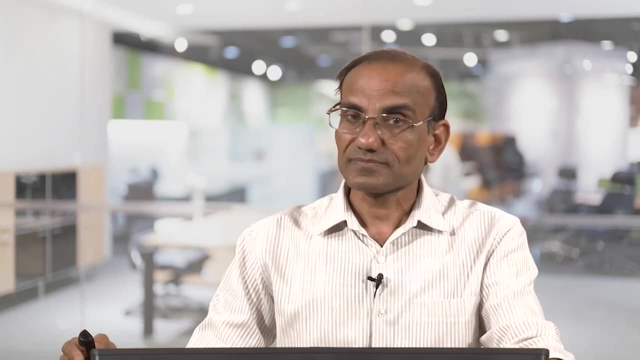 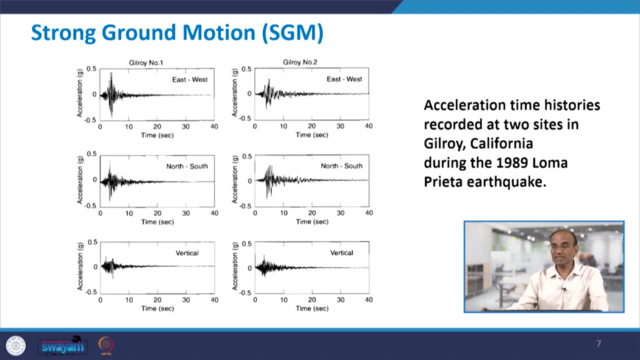 In practice, the rotational components are usually neglected and three orthogonal components of translation motions are more commonly measured. This is one of the example of strong ground motions which has been recorded at two sites which is located in Guadalajara, California, during the 1989 Loma Prieta earthquake. 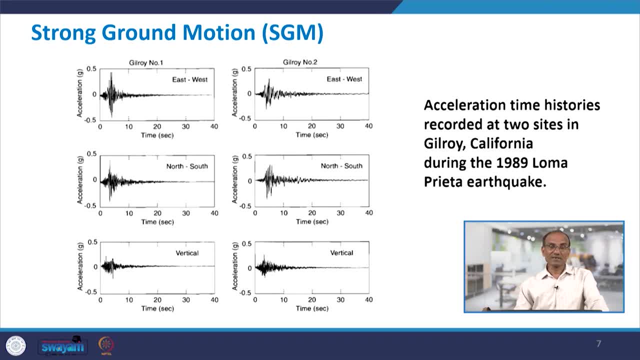 So during this earthquake, Gilroy number one and two, there are little difference in the site. First site is on the rock while the second site is on the soft soil. So you see the acceleration time history. then for the, for the, all the, both the sites three: 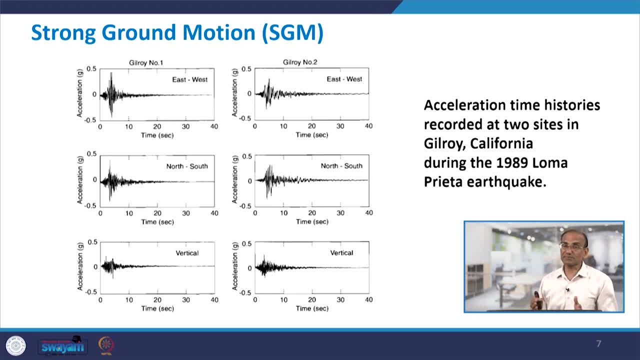 acceleration time histories are there actually, and these representing three translation components of earthquake motion in terms of acceleration time history. Okay, So in case of acceleration time history, on x axis you have time which is varying in seconds and on y axis, you have acceleration which is normally represented in terms of. 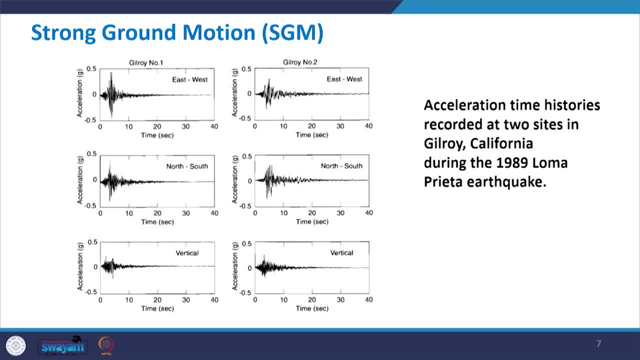 g, that is the acceleration due to gravity. So if you see it here that this is the acceleration due to gravity, so it is represented in terms of g. So 0.5 g, where 1 g, you already know, is nothing but 9.81 meter per second square. 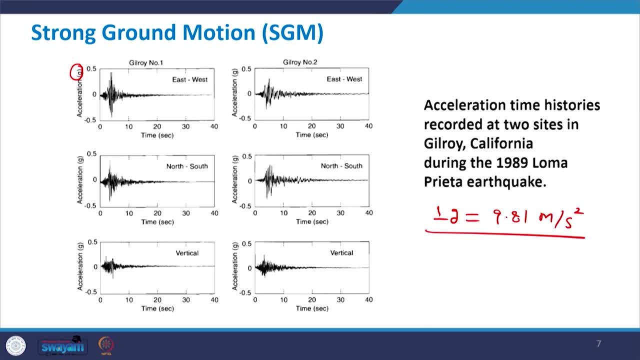 So again, the acceleration time history is in terms of gravity. So according to the acceleration dos 케kay, it here capacity and the acceleration time. So in terms of acceleration, here what you have for both the sides, 3 components of acceleration. 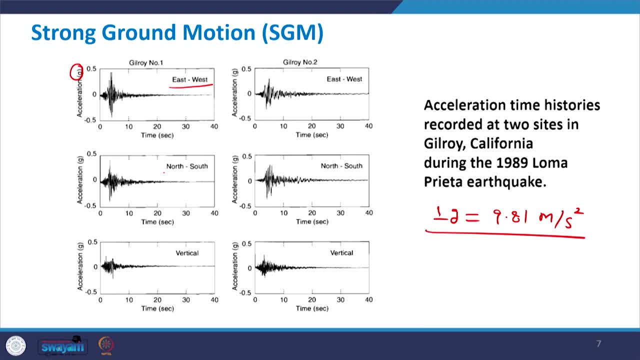 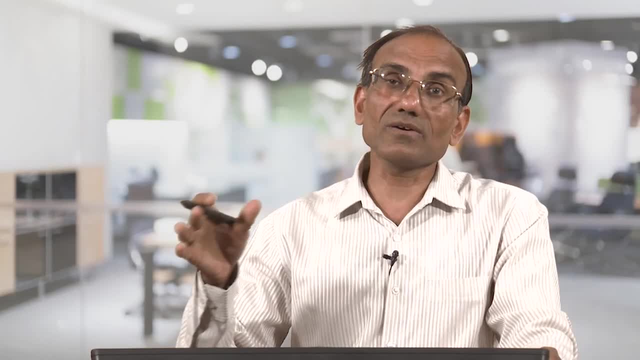 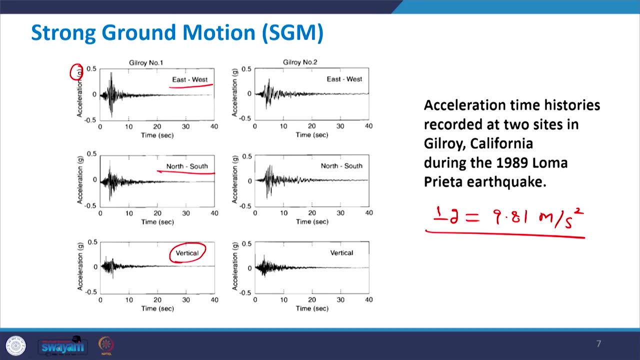 time history. first one is east-west component, north-south component, so east-west component and north-south component, they can be said in general lateral or horizontal components, while third one is vertical component. so all 3 components together describe the completely. 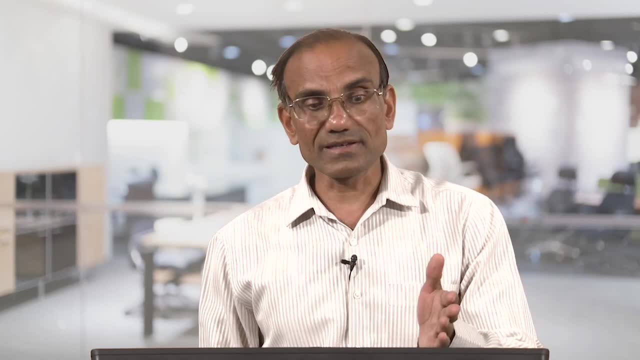 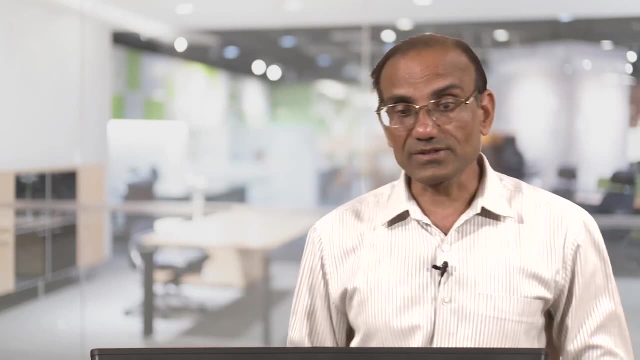 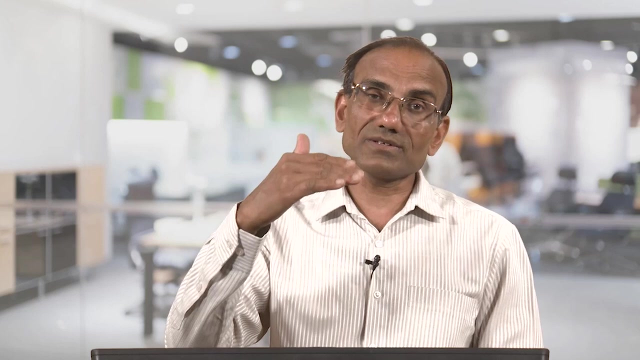 the earthquake time history, and this is for Gilroy number 1, as well as for the second sides also. So now what you see in these records, that the values are very much fluctuating. they are initially, like you know, starting from 0 and then they start reaching the some peak. 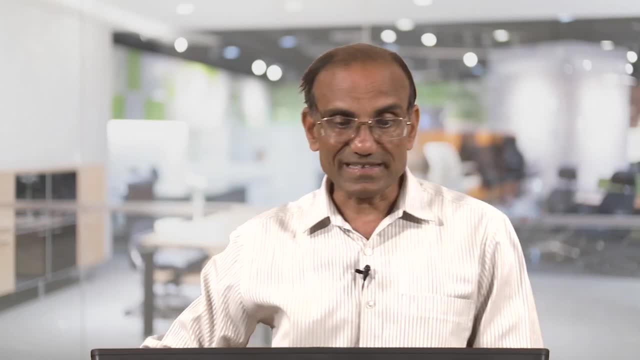 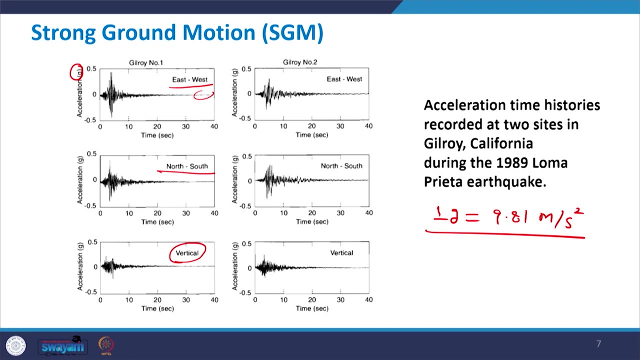 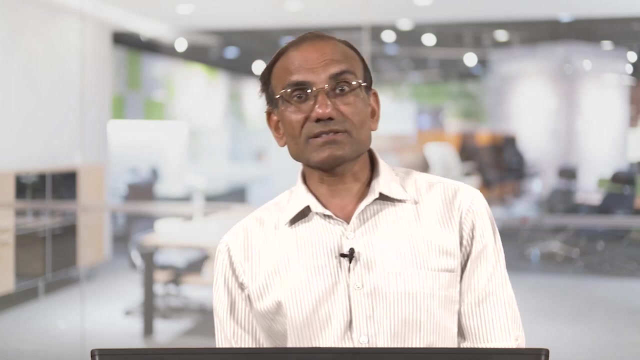 value and after the peak again start decreasing. at the end again, it becomes almost 0 after certain time. So when it becomes 0, that is the like, you know, kind of a duration of the earthquake, which we will discuss in detail later. Continue with this strong ground motion measure, then. what are the techniques for the measurement? 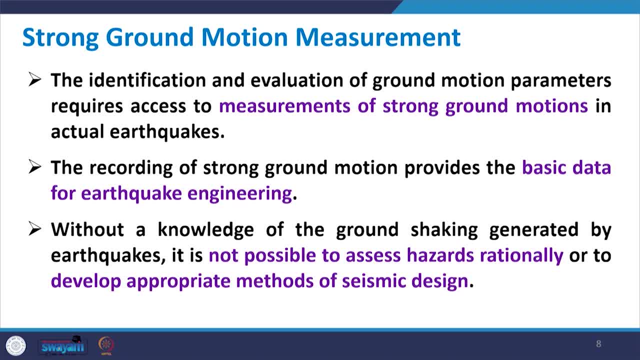 So the identification and evaluation of a strong ground motion parameters. it will require some measurements for actual earthquake and the recording of a strong ground motions provide some basic for earthquake engineering and without that knowledge of the ground shaking it is not possible to access a hazard rationally or develop appropriate methods for seismic. 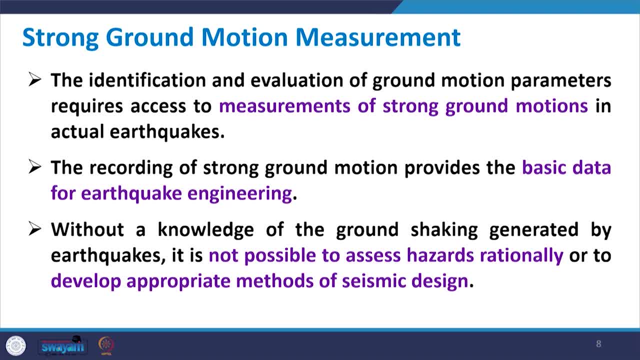 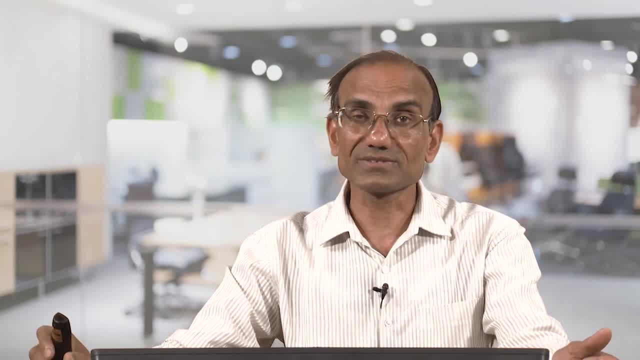 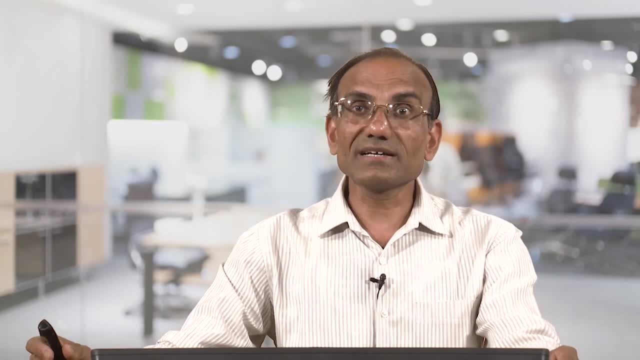 designs. So we need to measure what is the strength of the ground motion, strong ground motion, and then accordingly we design our structures or foundation for so that they can see the earthquake and they can survive. Normally they are measured relatively weak ground motions are measured by the seismographs. 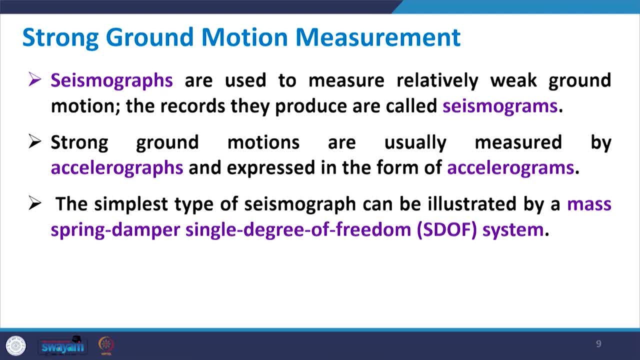 and the records they produce are called seismograms. So here there is one controversy: seismograph is not a graph, rather seismograph is one instrument which measure the earthquake record. rather the earthquake record is called seismogram. So so I think this should be. 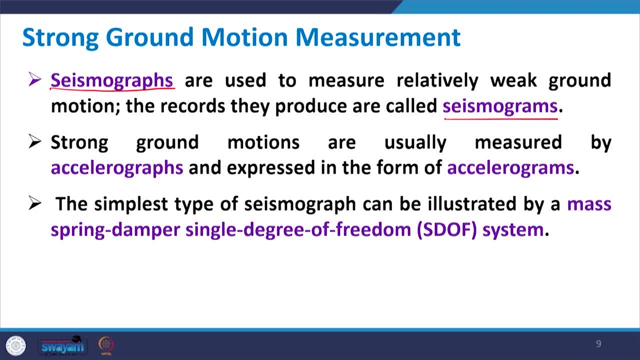 Okay, It should be clear. the seismograph is an instrument which measures. so when you use for measurement for the relatively weak ground, we use seismographs, but for a strong ground motions- normally they are measured what we called axelographs, because our objective is to measure acceleration time. 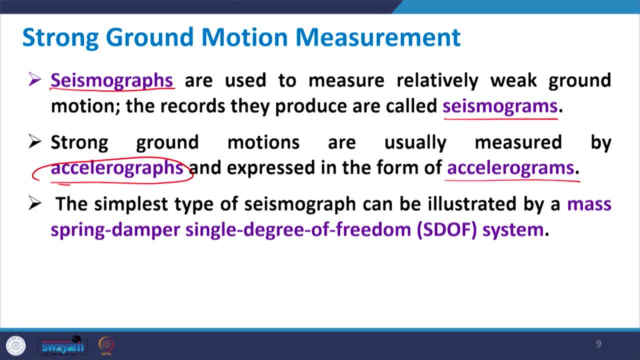 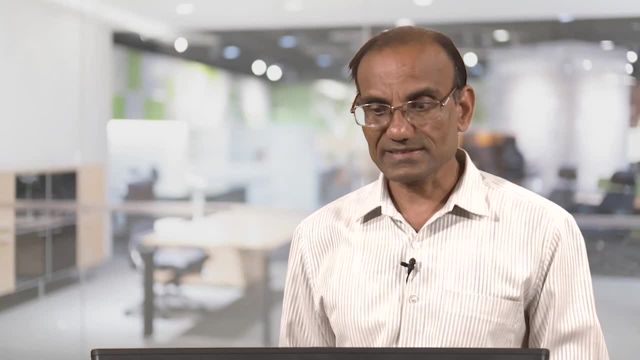 history, which is called axelograms. The simplest time of seismograph can be illustrated by what we call the single degree of freedom system, Which consists of a mass spring and damper. So let us. what is this next here? this is like like this, taken from the Kramer and, as I mentioned, 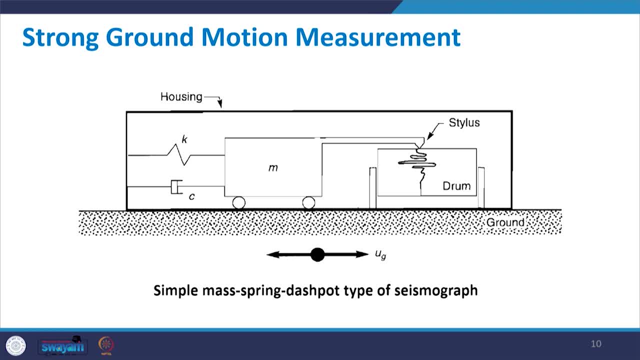 that earlier. also the quite like this. much of the things are from the Kramer's book here. So here what you have. this is simple ground motion measurement, which is like single degree of freedom system. what do you have in this system? you have a mass and you have stiffness. 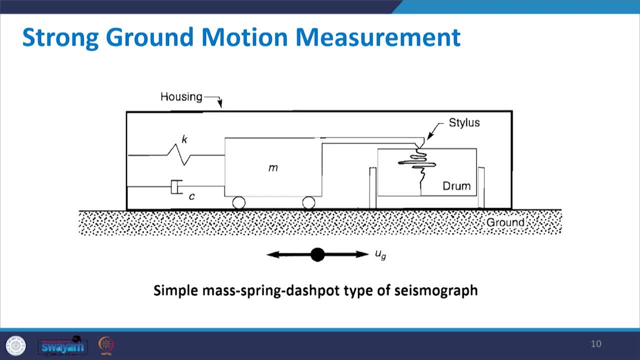 K and C. So this is basically single degree of freedom system. what happens? this mass is situated on the roller. this this is. you could see that there is a roller, so two rollers are there. So what will happen when earthquake wave comes in the lateral direction roller will. 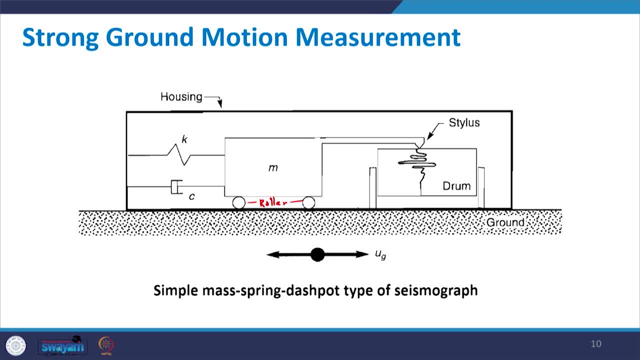 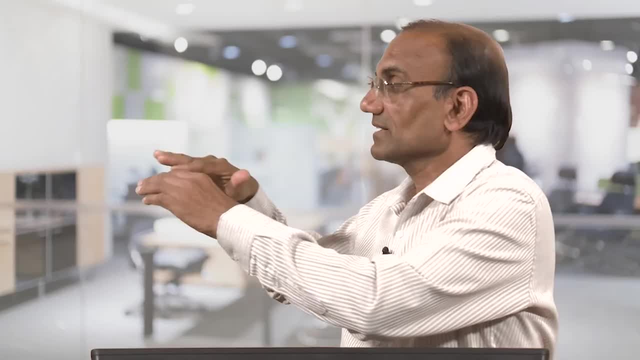 mass will move like this. as a result, this attachment will move like this: Okay, Okay, Okay, Okay, Okay. So it will move and there is a drum and this drum is vertically moving. So it is like this vertically drum is moving and on this moving drum. 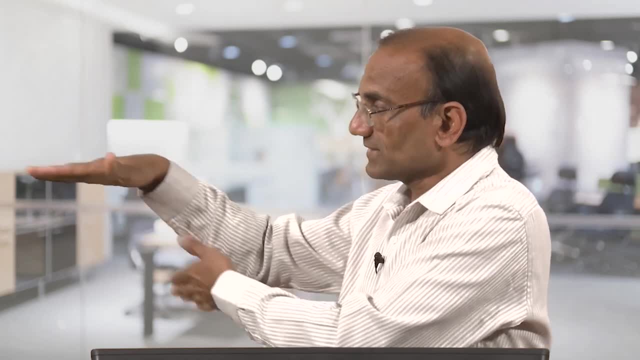 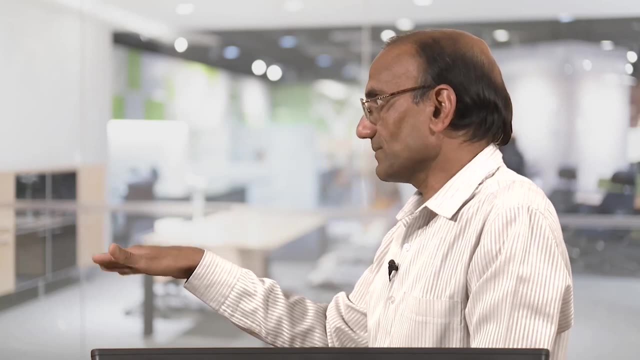 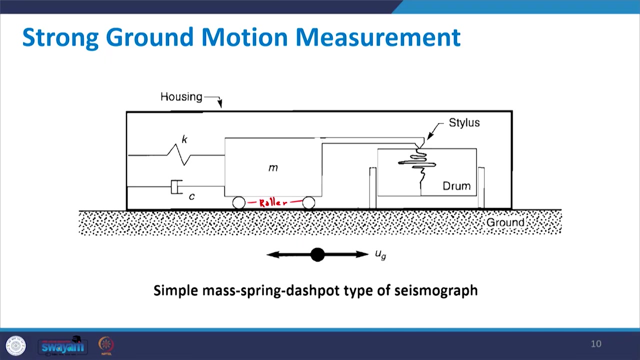 You have this pen which which will mark the wave when it moves like this. So it will, because due to the vibrations- earthquake vibrations- it will go like this and it will record while drum is moving. So this is the case. So this is the normally the earlier one. 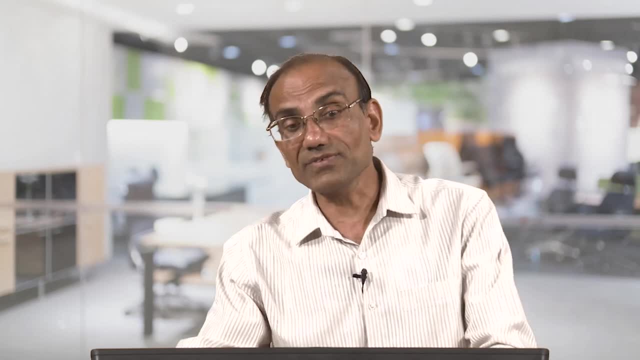 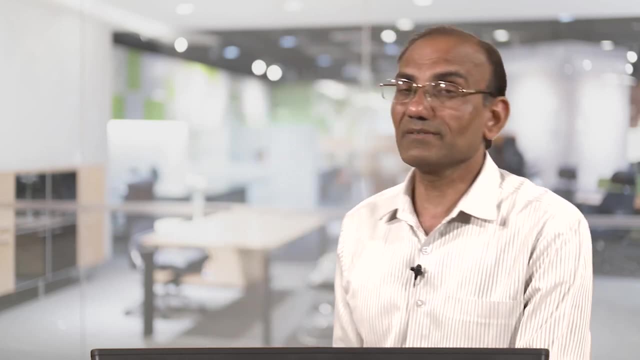 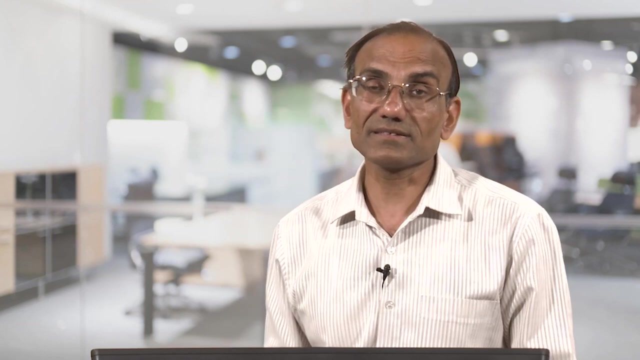 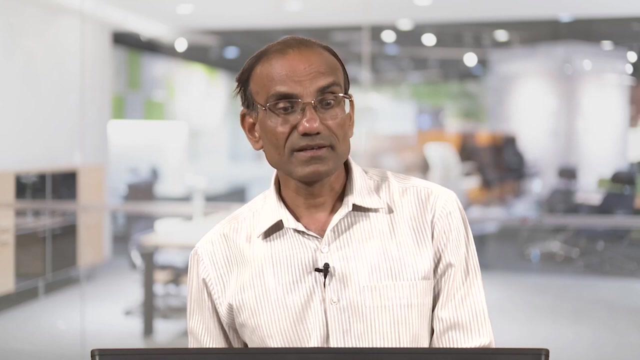 when the digital was not there and usually the first kind of seismograph was like this. So that has been invented and it has gone quite long time, and successfully. they are, you know, quite like a. as I mentioned earlier, that first engineering record of earthquake was during 1940: El Centro earthquake. 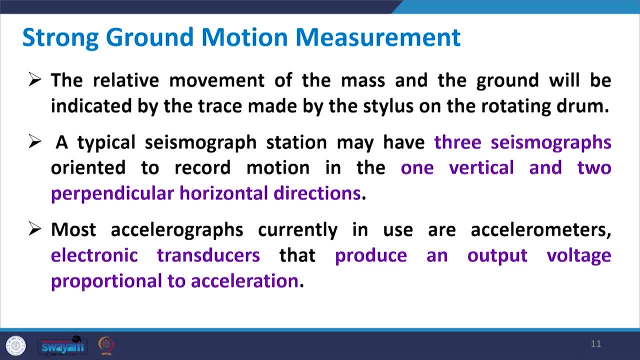 Continue with this. the relative movement of the mass and the ground will be indicated by the stress made by the stylus on the rotating drum. so, which is we already discussed, And a typical seismograph have three seismograms oriented to record motions, to the one vertical. 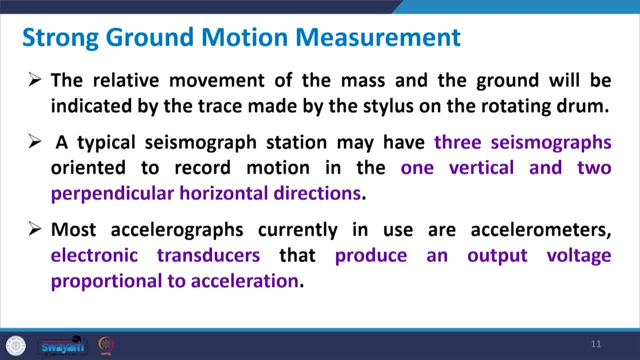 and two perpendicular horizontal directions. Most accelerograms currently in use are accelerometers and some transducers that produce in terms of output, In terms of voltage, which will be proportional to acceleration. that means there is a variation in the voltage and when acceleration increases, so voltage will be high. 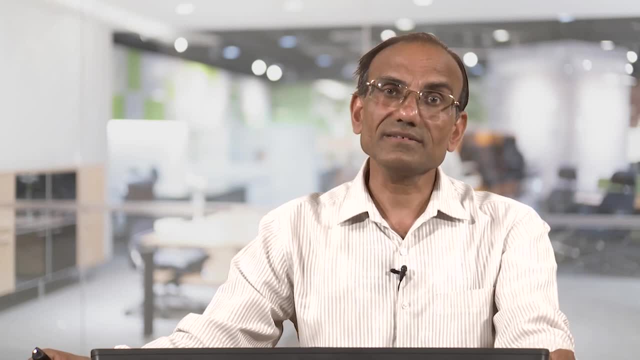 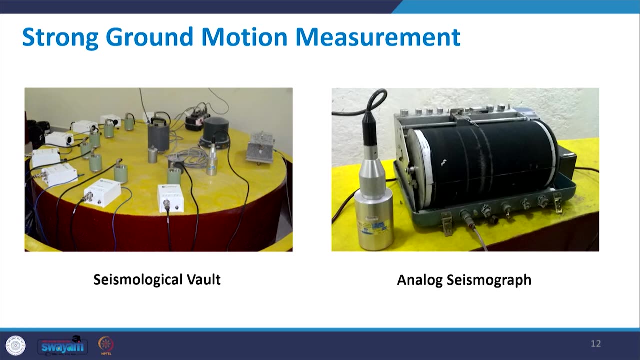 Strong ground motion measurements are here. so it is. you could see here: on the left hand side it is seismological vault and on another side it is analog seismographs. both of these photographs are taken from our Seismology Observatory located in Department of Earthquake Engineering at IIT Roorkee. 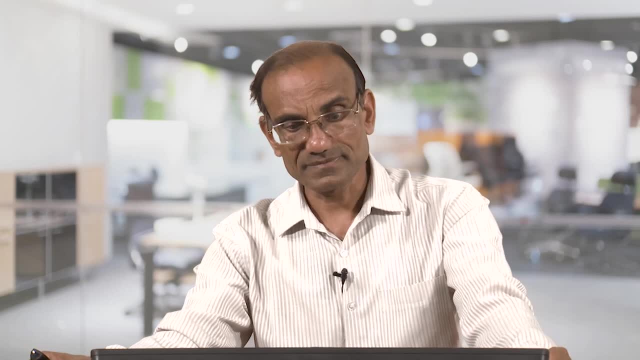 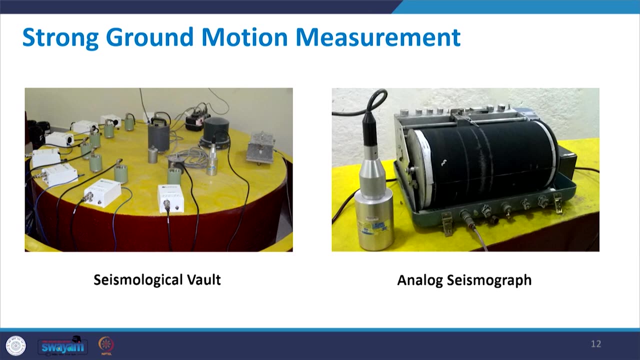 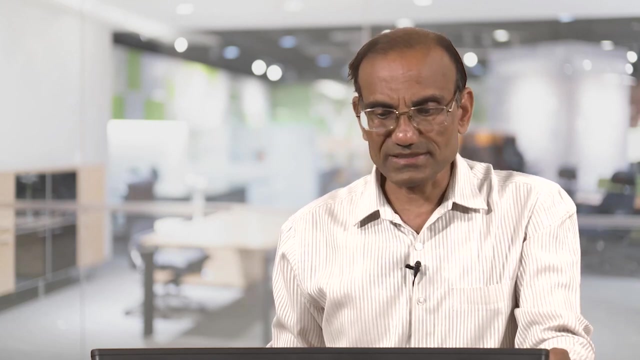 So this is from our own lab, department's lab. So there is a vault and at the bottom there is, you know, that base on the top of like kind of a rock, instrumentations are done, which is normally you call sensors, and on right hand side a zoom picture of one of the instrument. 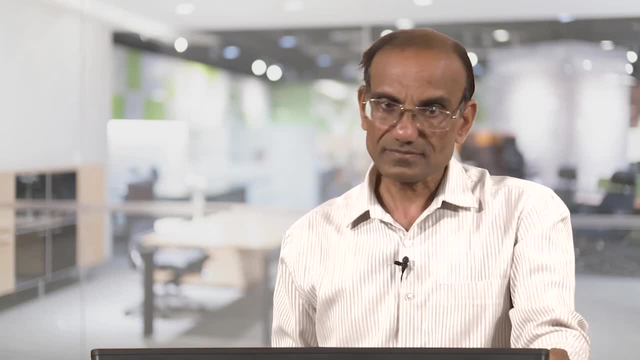 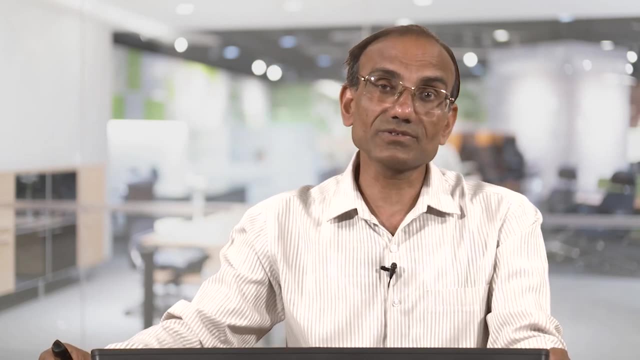 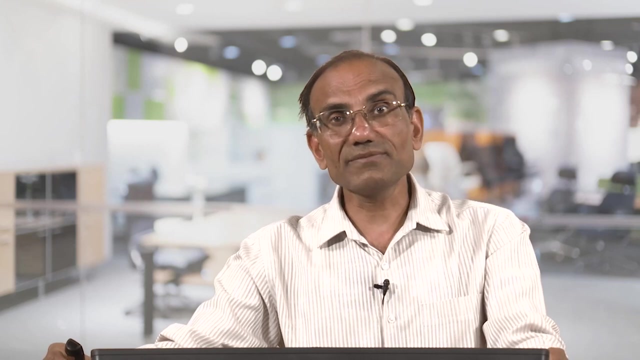 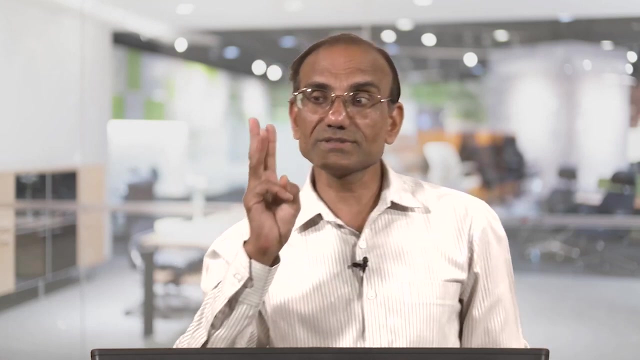 Analog seismogram is shown. Now it is time to characterize the SGM. SGM stand here for in the short, strong ground motion For engineering purpose. it is important that we characterize the earthquake motions. and when we characterize earthquake motion, they are done normally using three parameters. 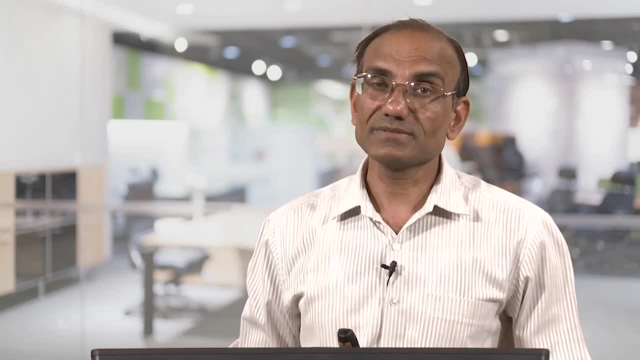 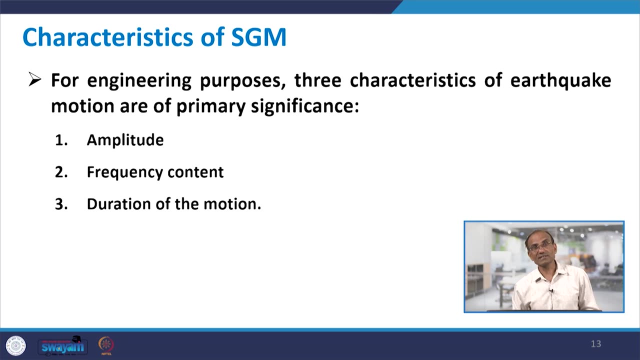 What are the three parameters? First is amplitude of the earthquake, The motion which is indirectly measuring energy content. then you have frequency contents. how frequently, like you know that with the time the motion like it is changing, the peaks and troughs are changing. that will be coming in frequency, content and duration of the motion. 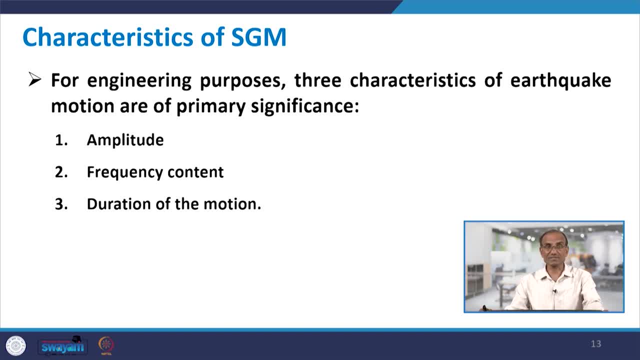 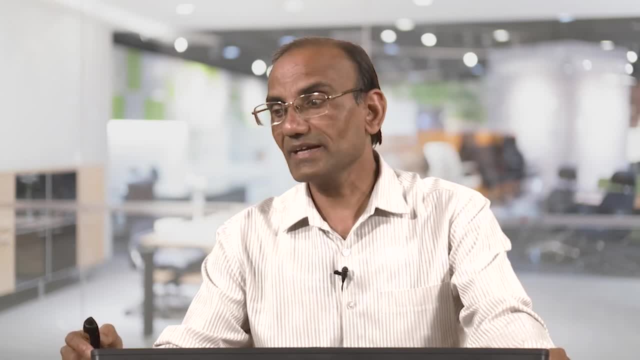 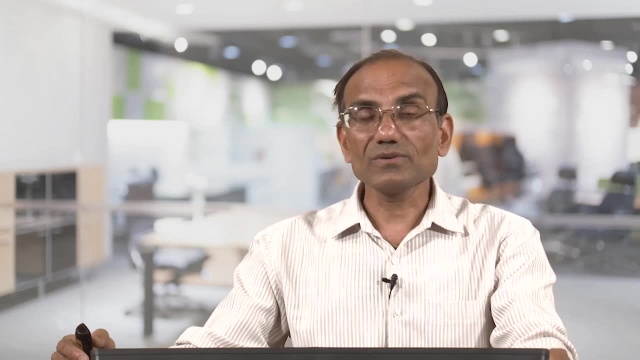 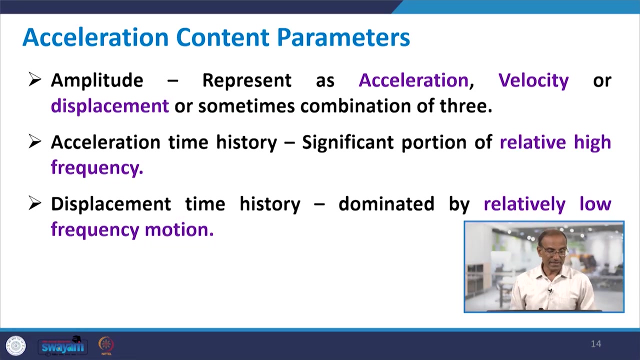 that means for how long the earthquake duration lasts. so these three parameters together can help to characterize SGM- Strong ground motion- and in the next slides we are going to characterize these. we are going to discuss one by one each. So normally for amplitude, acceleration, content parameters are used and for acceleration 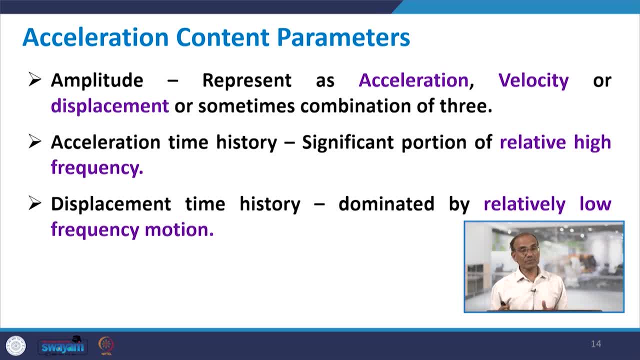 you have amplitude which represent and acceleration, and it can be represented by amplitude, can be represented by either acceleration velocity- Okay Velocity- or displacement. Similarly, acceleration time is here. there is one difference: when you have acceleration time history, then significant portion of that time history is normally in high frequency. 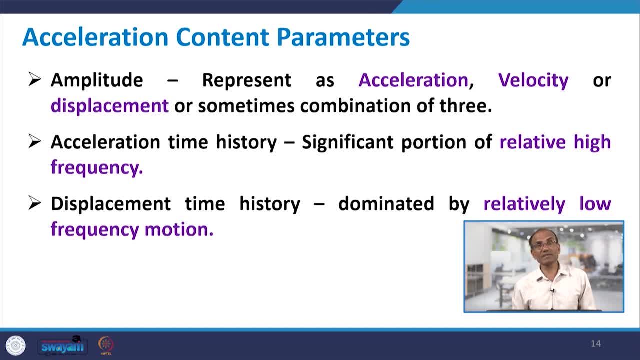 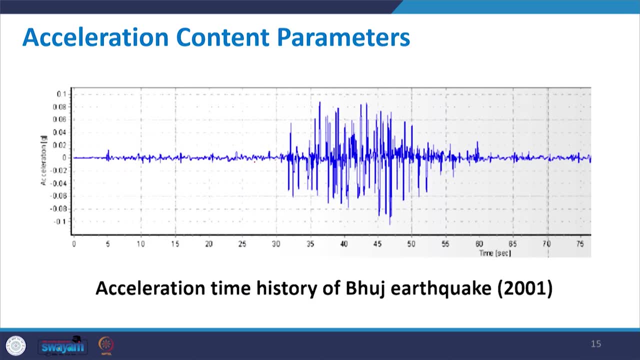 range, while for displacement time history it is dominated by relatively low frequency motion. So for high frequency acceleration time history will have large portion for that, while for displacement time history, For example, this is one of the acceleration time history from earthquake of 2001 and this 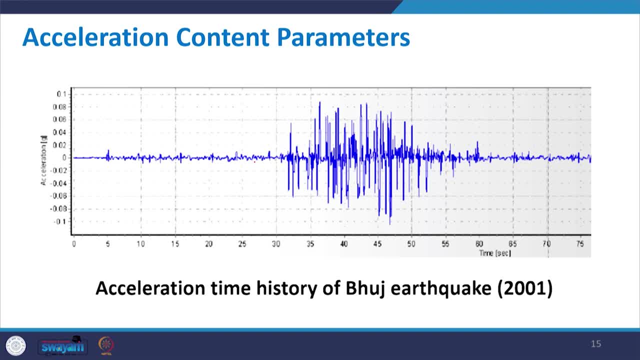 is lateral component. what you could see: on y axis there is a acceleration and on x axis you have time. so this is record. is was lasting about 75 seconds, but you could see the signals are very weak. up to 30 seconds- Initial 30 seconds. 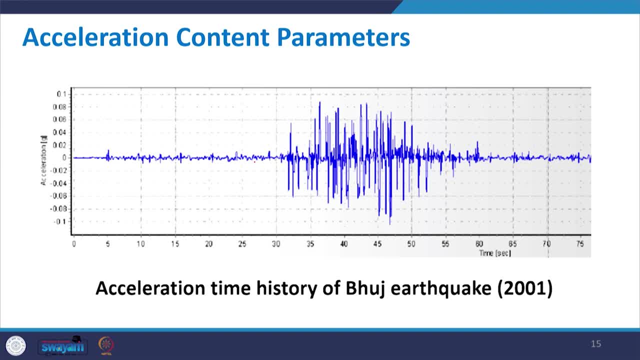 Okay, The peak values are very low, but after like around 32 seconds it all of a sudden jump and you get some peak values around 47 seconds here. Here, when we talk about peak, our meaning of the peak is absolute peak. 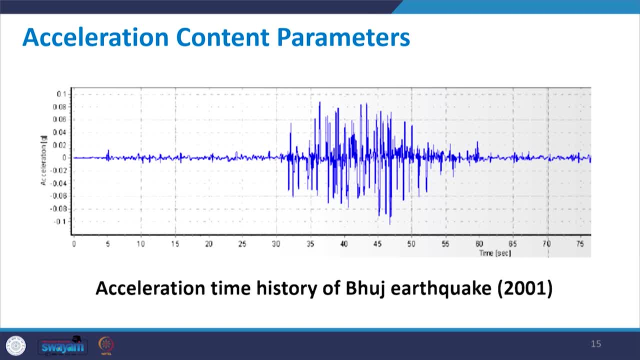 It does not matter whether it is positive side or negative side Here. in this case the maximum value is more than 0.1, but that is happening towards the negative side, So the peak will be here, not this side. Okay, 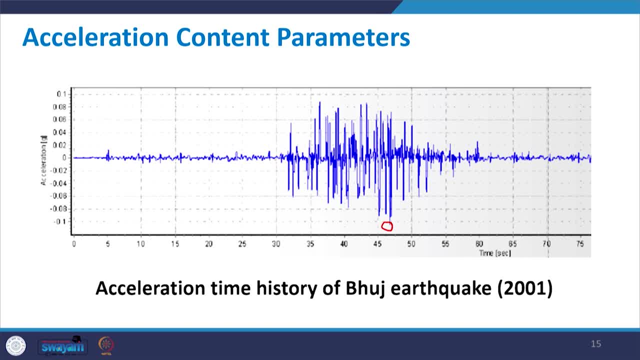 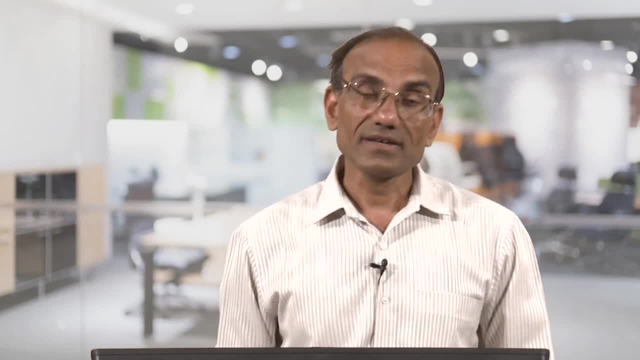 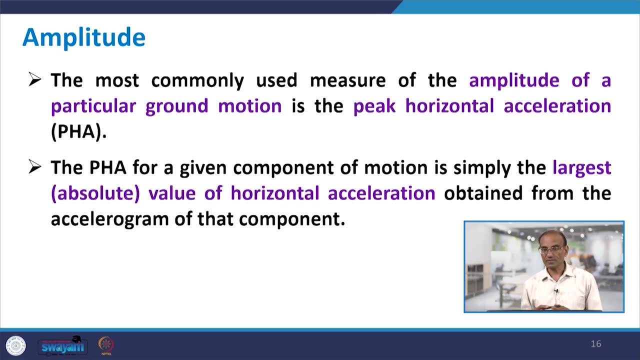 So, irrespective of whether it is positive or negative, we say: Now we collect the peak values and then we further process. So what is done for the amplitude? The most commonly used measure of the amplitude is called for, particular the peak horizontal acceleration, PHA. 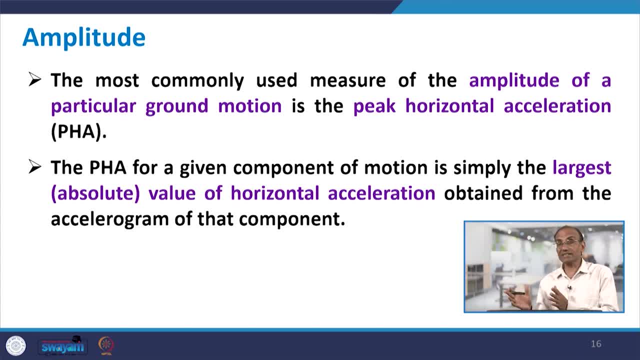 So it is saying the acceleration in the horizontal direction, the maximum value of the acceleration in the horizontal direction will be treated as a PHA, And the PHA, for given more component, is simply the largest absolute value of horizontal acceleration. Here absolute means simple, that it can be on the positive side or negative side. 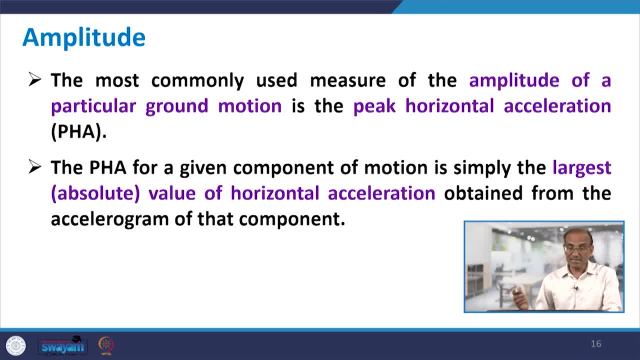 Here one thing I will most of the time instead of PHA. many times PGA is used, and you would have come across many times what is called PGA, which stands for simply peak ground acceleration. peak ground acceleration, Okay, Peak ground acceleration. 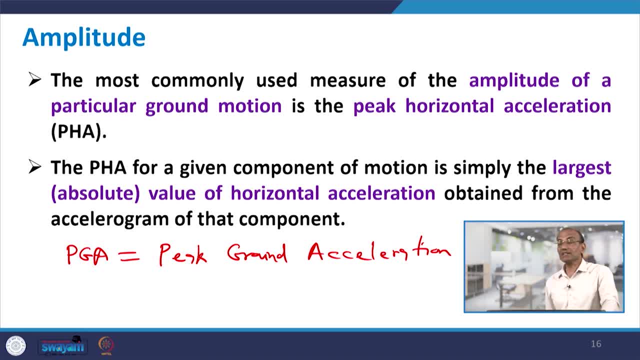 And this is the term widely used- PGA. Here, instead of PGA, we are using PHA, because this is like more clarity. When we write PHA, it is very clear that this peak will be in the horizontal direction, But PGA could be either in the horizontal and vertical direction. 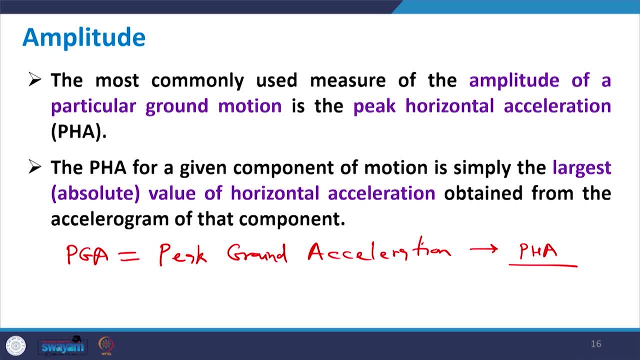 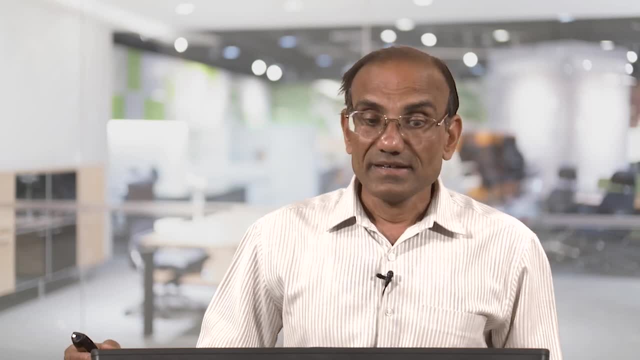 However, if nothing is written with the PGA, then it will be considered that it is in the horizontal direction. Okay, Okay, So the value in the horizontal direction is more important than in the vertical direction. So we will. that we will discuss later again. 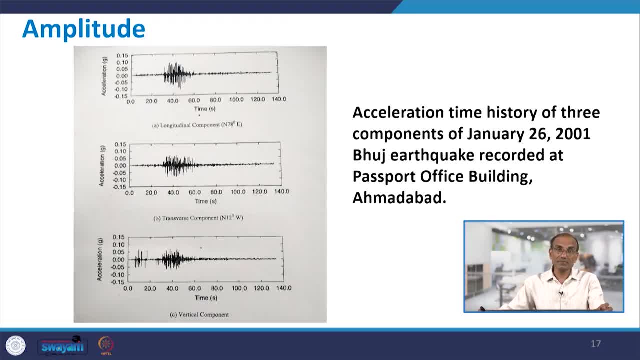 In this slide you have three components of 2001 Bhuj earthquake, which occurred on January 26.. And and the record taken was at the Passport Office building in Ahmedabad. And this record is taken by Department of Earthquake Engineering at IIT Roorkee using 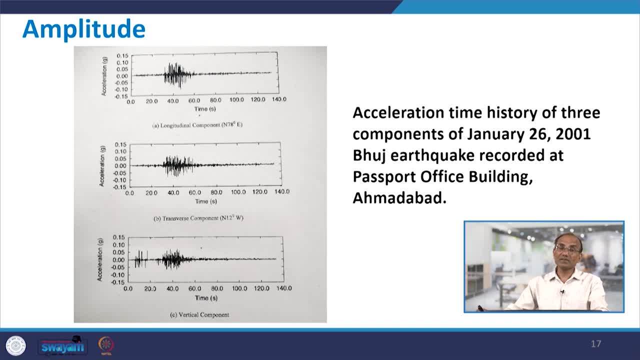 our instruments And what you see. Okay, So you have acceleration time history On the top. you have longitudinal components, Then you have transverse components. So first, two components are: both are horizontal components and third, one is vertical component. 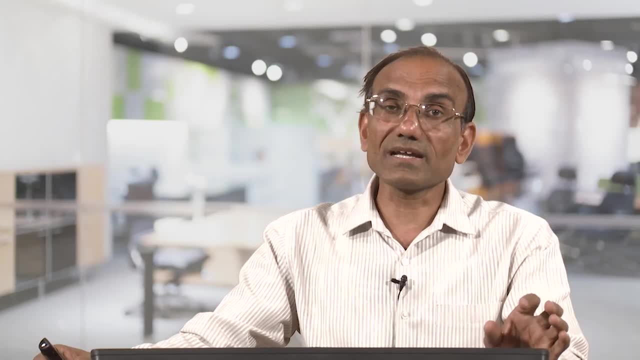 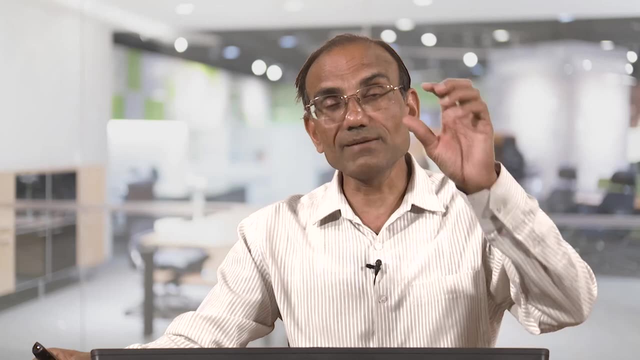 Normally vertical components, values, peak values, are less than the two horizontal component, which you can see here in both the figures, that the values, that is, the amplitude, is less. And out of these two longitudinal component or transverse component you have two horizontal. 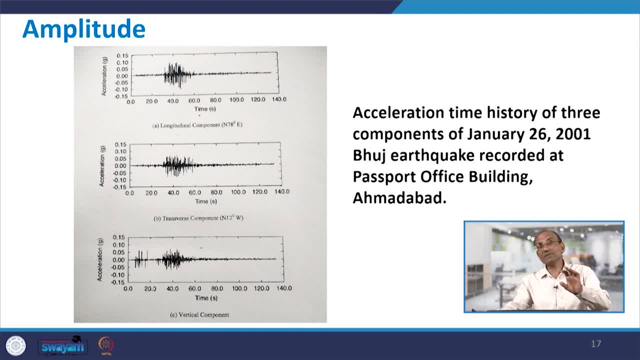 components, Whichever is, give you the higher peak value. we consider that for determining PGA or PHA. So here you could see that the top one have little higher values, which is here about, as we discuss, are going about 0.1, but the here it is less than this. 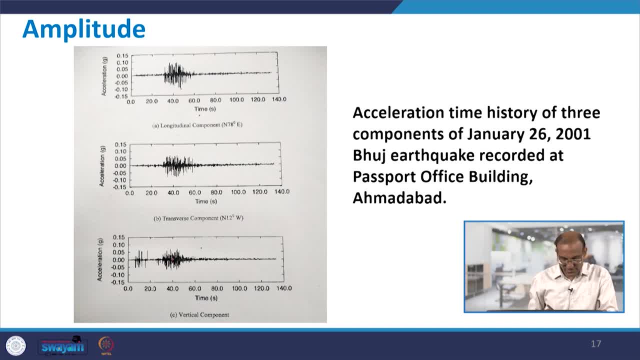 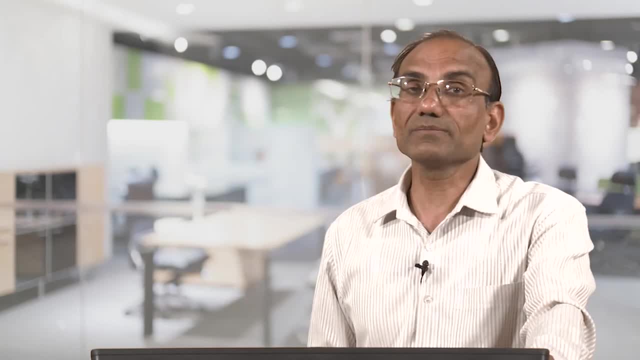 So here, maximum value is around 0.7, and if you go for the vertical, the left, it is around 0.05 only. So this was about 0.1.. Okay, Okay, So these are the records obtained from the Booz earthquake. 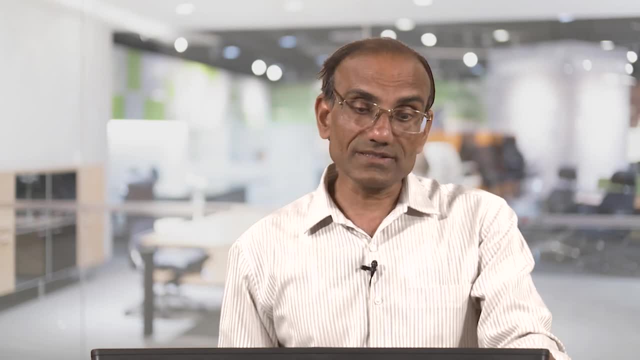 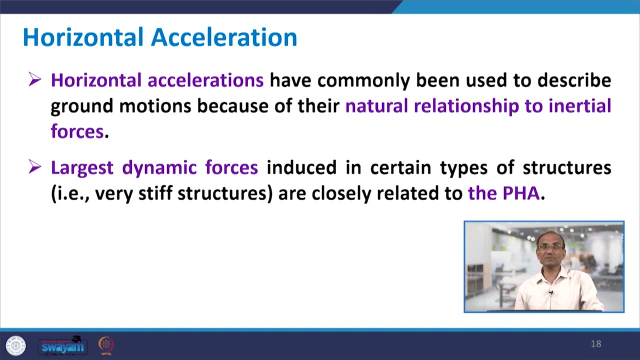 Continue with that. we further explore what is in the horizontal accelerations. They have commonly been used to describe ground motions because of their natural relations to inertial forces, Because inertial forces will be governed by the horizontal acceleration. Basically, for inertial forces will be simply mass multiplied by the horizontal acceleration. 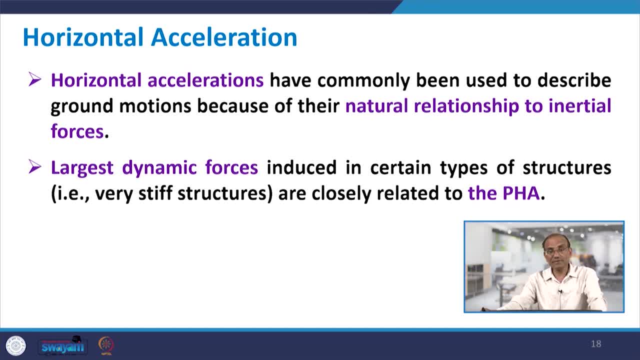 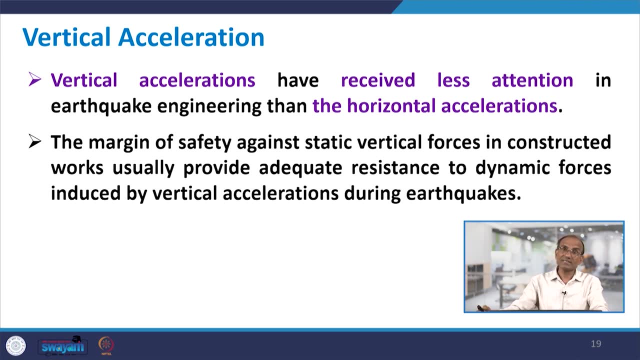 So that is why this is important And largest dynamic forces induced in certain types of structures- that is, very stiff structures- are closely related to what we call the PHA Peak Horizontal Acceleration, For vertical accelerations have received less attentions in earthquake engineering than 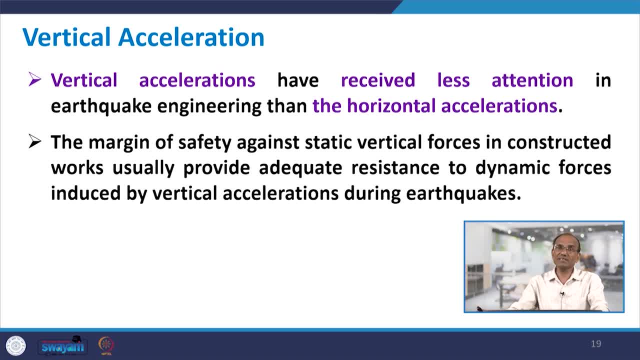 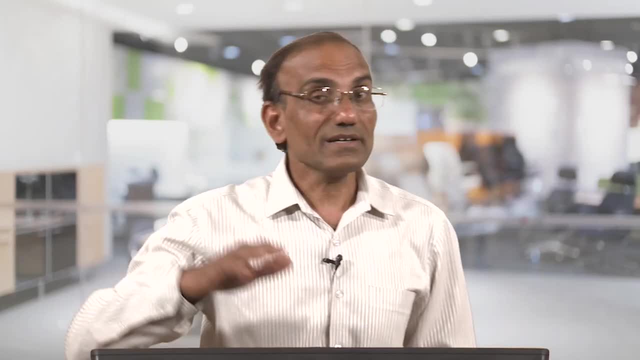 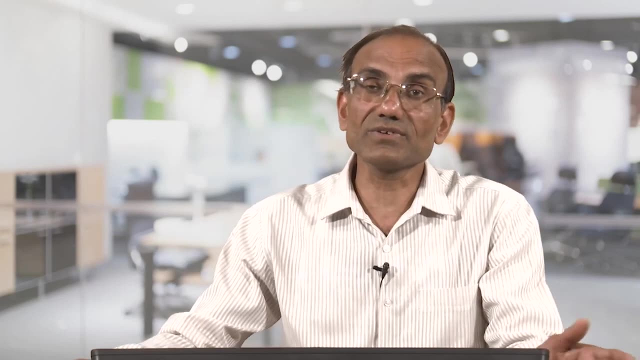 the horizontal accelerations And the margin of safety against static vertical forces in constructed works provide adequate resistance to dynamic forces induced by vertical acceleration during the earthquakes. So basically what it says. you know why this, like for earthquake engineering already. if the structures are designed for a static load without earthquake, also they are survive or 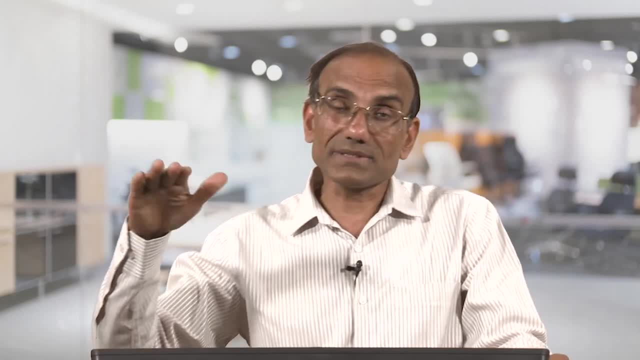 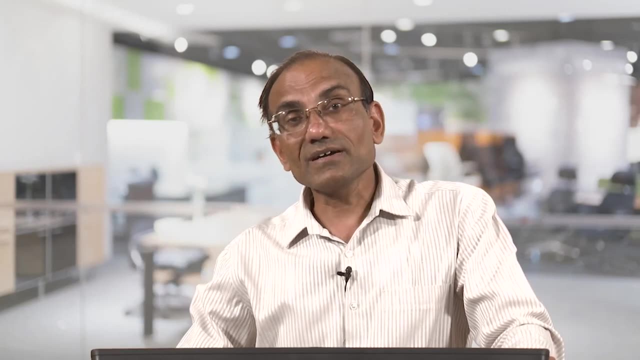 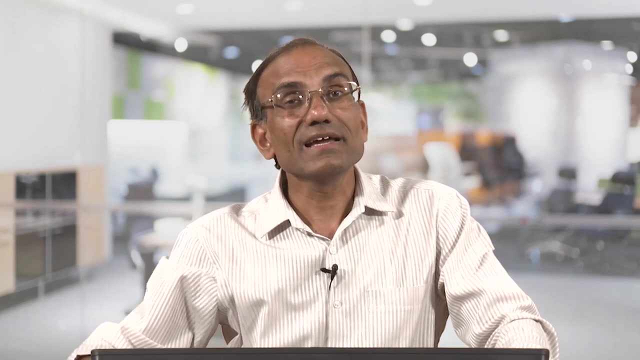 like without earthquake. like you know, their design is done, But what happens during the earthquake? there is a lateral component which, during the earthquake, it not only the vertical force but horizontal force is also applied and the result: most of the structures are designed only for vertical force because they are assuming there is no. 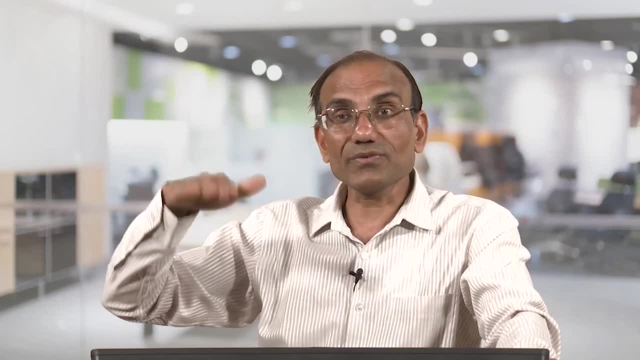 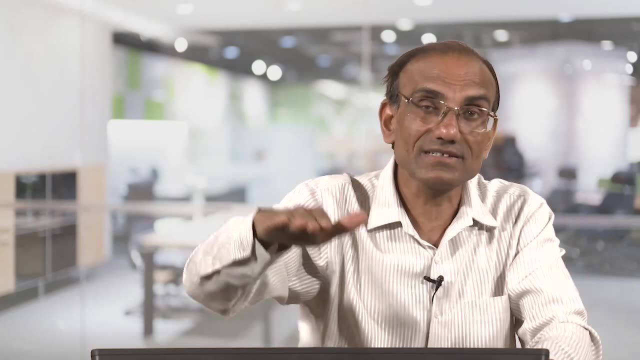 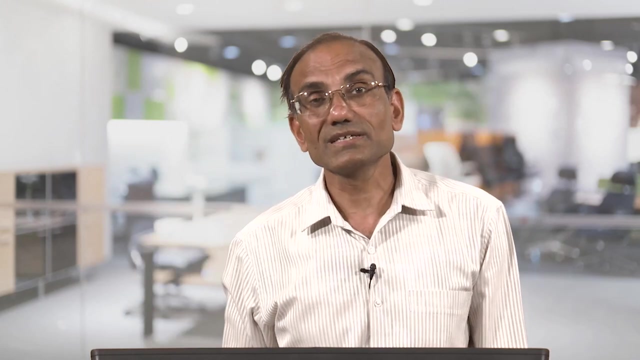 earthquake. So as a result, they can take the vertical force because they may have enough strength, but because earthquake also apply the force in the horizontal direction or the lateral direction and if your structure or building is not designed for that earthquake lateral force, Then it is going to be damaged. 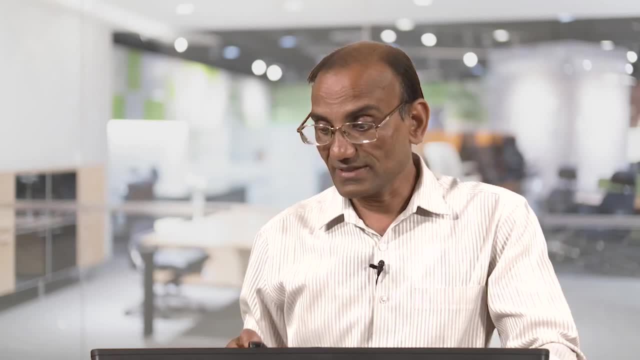 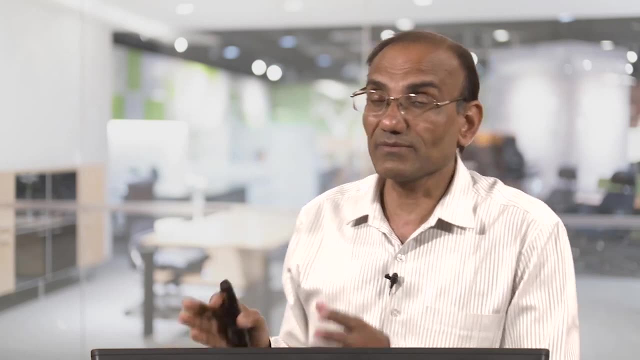 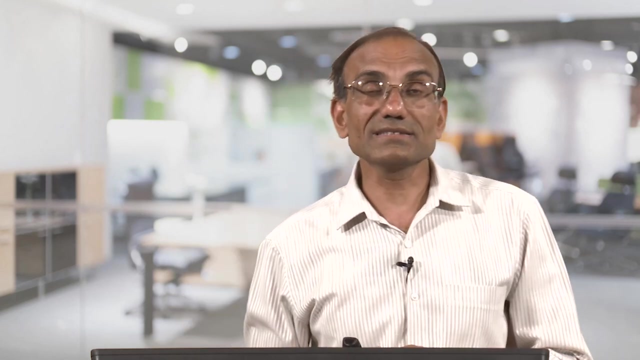 Or even it is going to be collapsed. So this is like. that is why, like again when we consider the earthquake, if we can consider all the three components, both horizontal and one vertical component, that is the best thing. However, for many analysis, for engineering purpose, only one component is considered and 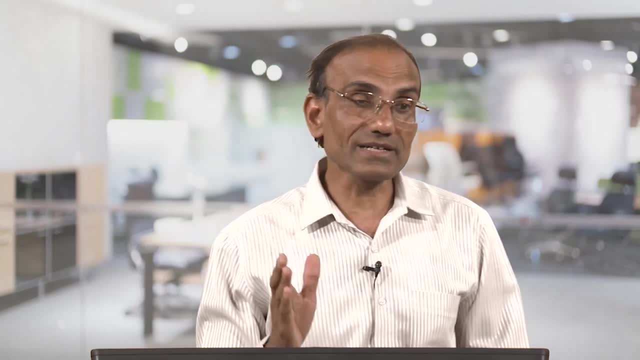 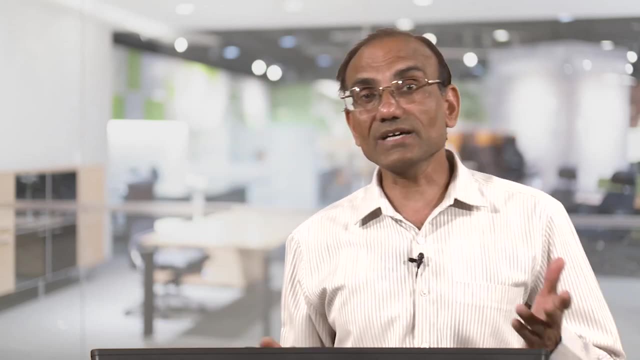 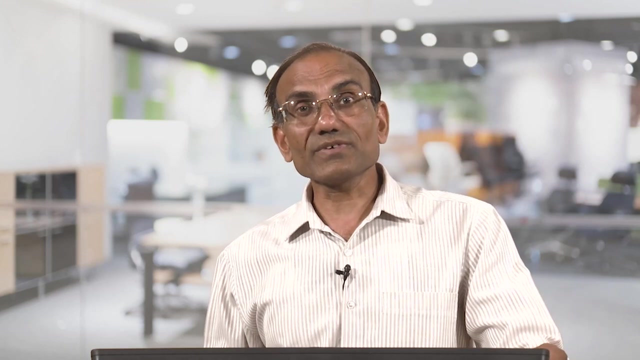 if you are going to consider only one component, then it will be the horizontal component, not the vertical component. and out of the horizontal component, which one we should consider which give you the highest value of Ps? Okay, So continue. the characteristics of a ground motion at a particular site depends on earthquake. 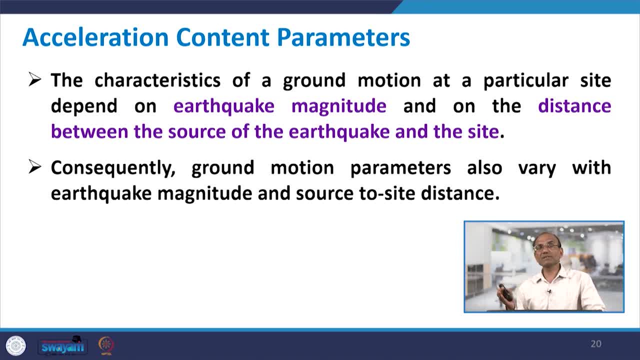 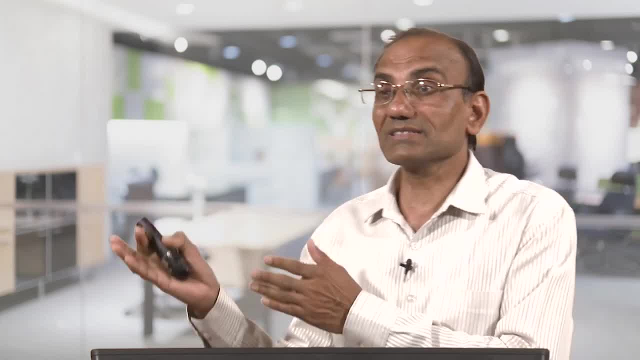 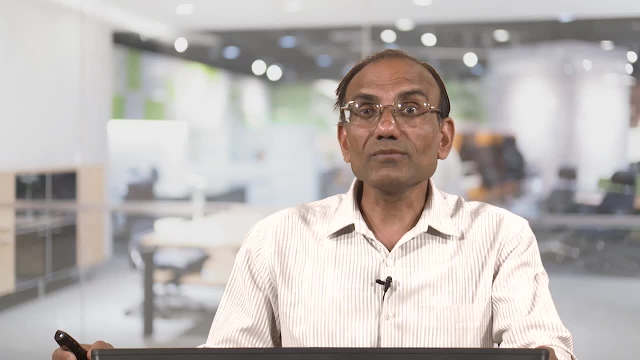 magnitude and on the distance between the source of the earthquake and the site. So how much is the magnitude and how is the? how far is the site from the source, that is, from the epicenter, basically? So, as a result, ground motion parameters also vary with earthquake. 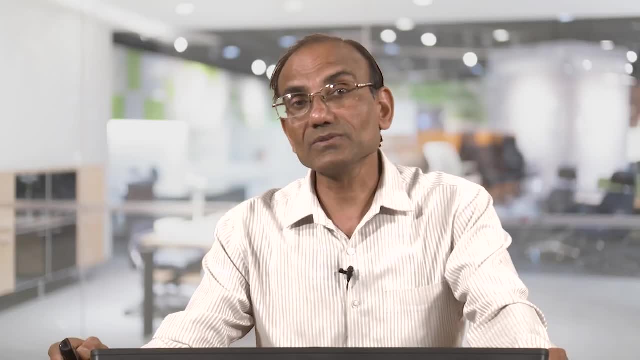 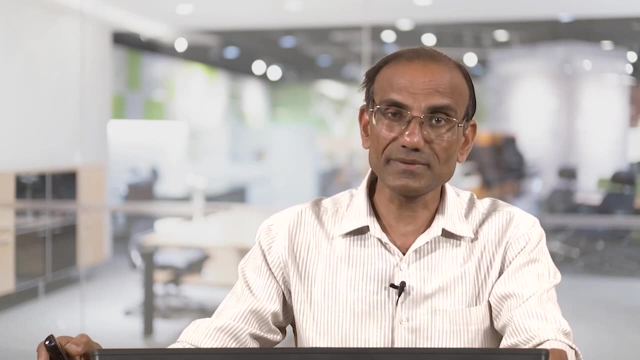 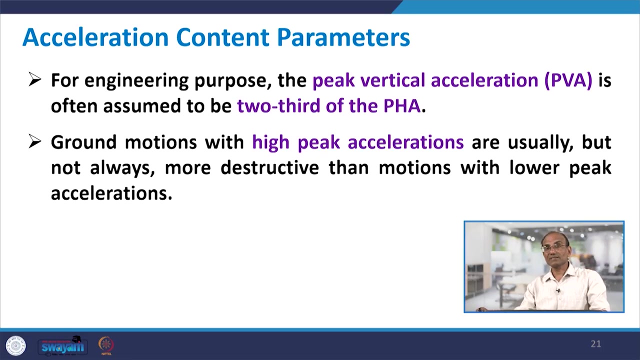 Earthquake magnitude and source to site distance. So that will be governing parameters. if earthquake magnitude will change, So this ground motion parameter will be expected to be higher. For engineering purpose the peak vertical acceleration is often assumed to be two-third on the of the PHA. 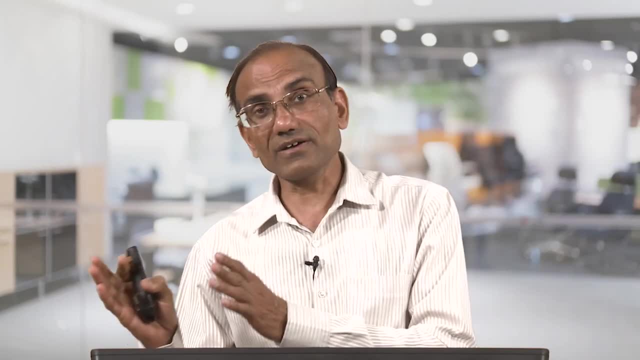 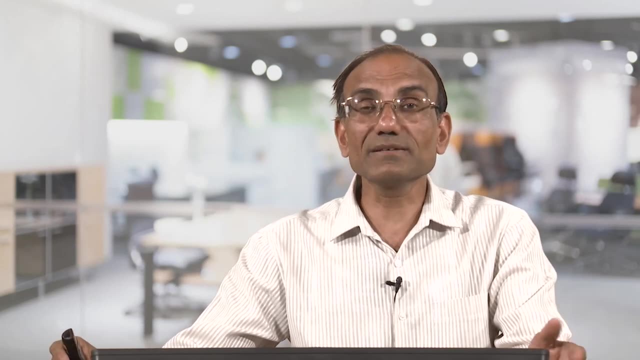 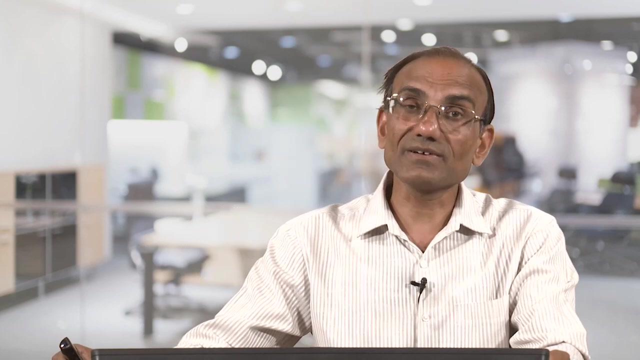 So if we have a single record, let us say I have a record of only peak horizontal acceleration with the time Time is two, Okay, And I do not have, like you know, the vertical and I simply I need to design for the structure for the horizontal load as well as vertical load. in that case, like our code, IS 18923 is. 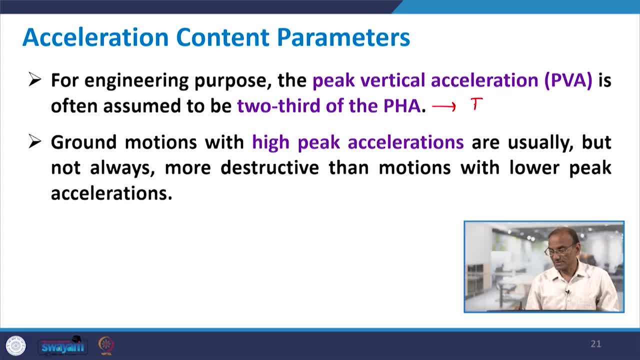 also suggest the same thing. So this is also suggested by Indian standard code IS 1893, which is the latest version is 2006. you can see the part one. So the same recommendation that vertical acceleration can be considered as two-third of horizontal one. 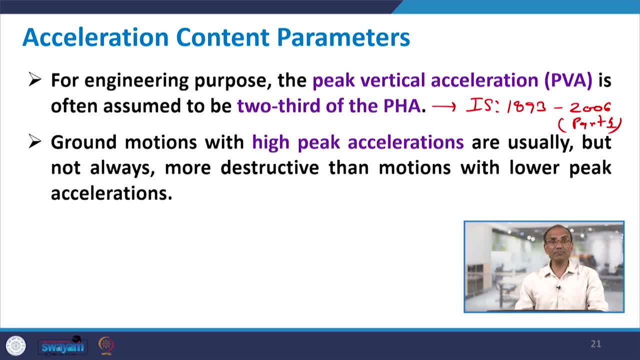 Ground motions with high peak accelerations are usually, but not always, more destructive than motions with lower peak accelerations. So naturally, if a peak acceleration value is higher, then it is normally more destructive, though it may not be the always, because it depends on other things like frequency contents. 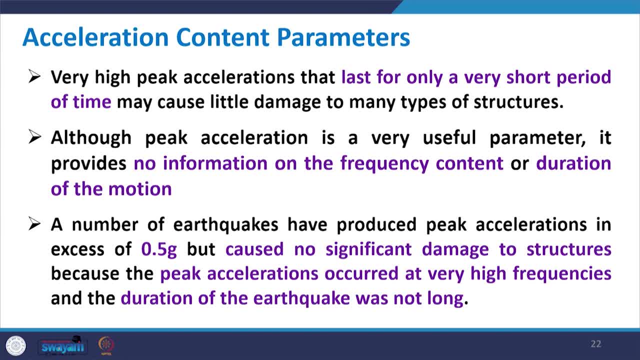 and others which we are going to discuss later, but most of the time this is the case. However, The very high peak acceleration Last only for a few seconds, only a very short period of time, and if time for which this is only for a very short, then it may cause little damage to many types of structures. 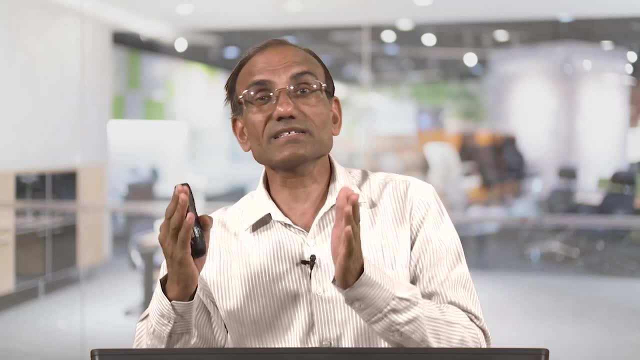 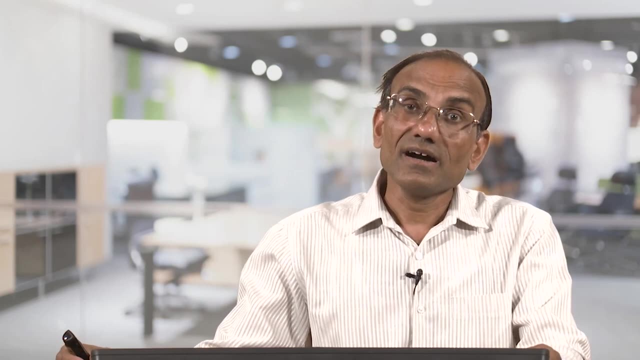 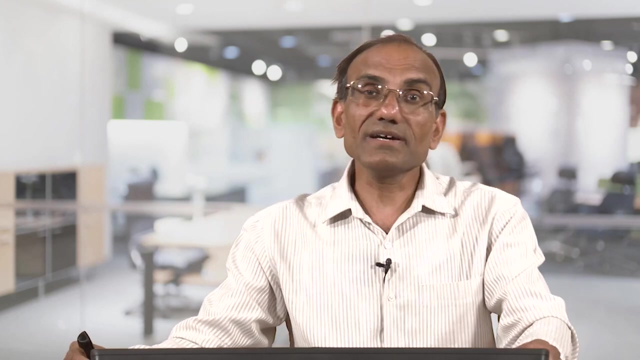 So it is also depends this peak value is sustaining. for how long it is for them like a fraction of seconds or few seconds. that is there, although is the peak acceleration. PHA or PGA is very useful parameter, Okay. However, it do not provide any information: the frequency, content or duration of the motion. 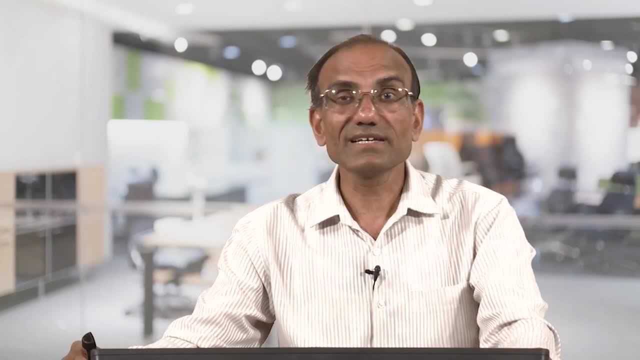 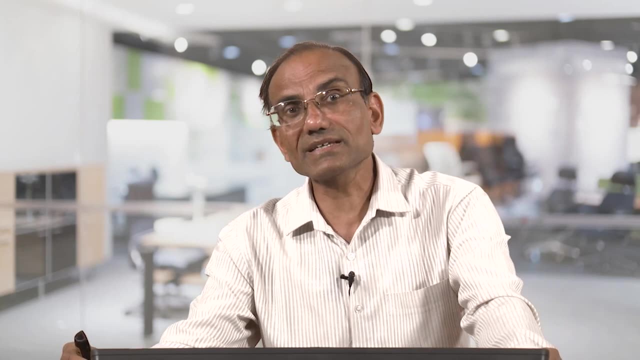 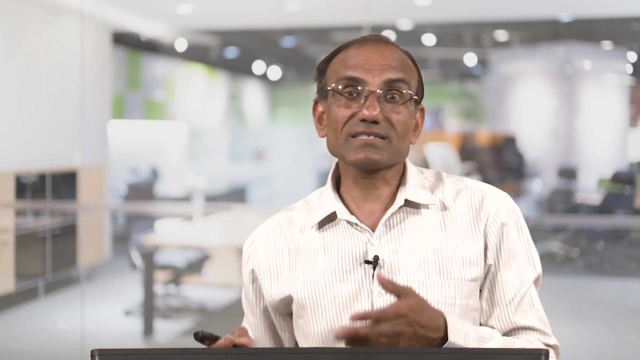 which the latter two come part, that is, frequency, content and duration, is also important when we design the structures. A number of earthquakes have produced peak acceleration in excess of 0.5 g. it has been observed in the past that the PGA value is going to 0.5 g, but still there was no significant 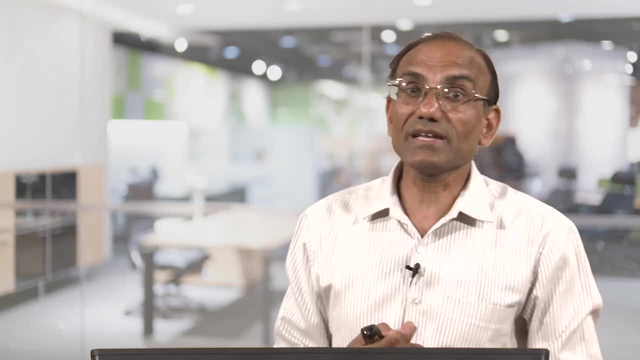 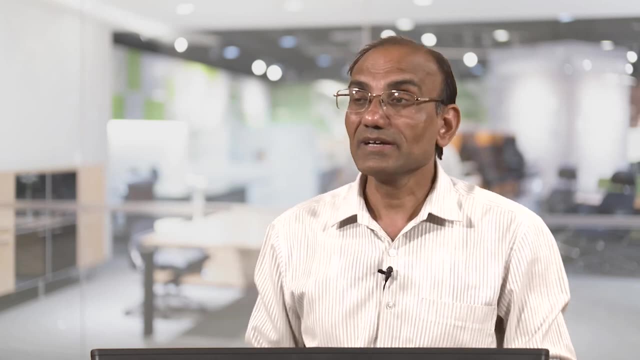 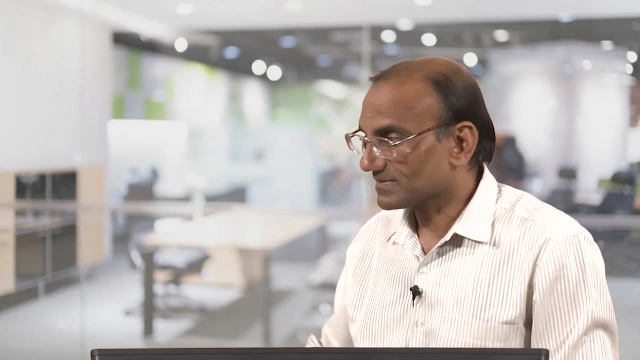 damage was done to the structures. and why? Because the value, This peak acceleration occurred at very high frequencies and the duration of earthquake was not long. very high frequencies means in few seconds, in a some time. it runs very fastly, So it move. you know the peak acceleration was there, but then it have come momentarily. 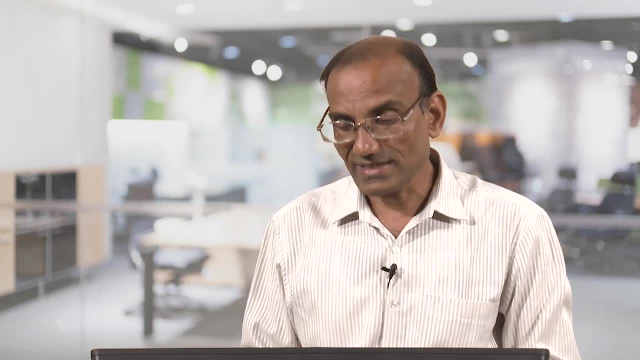 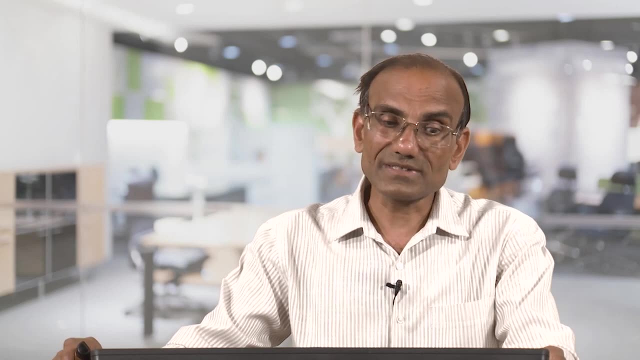 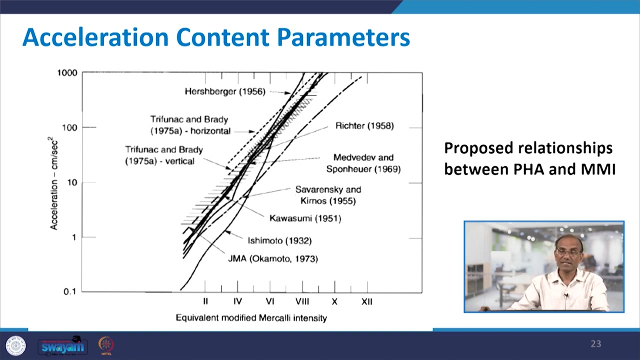 very like. you know fraction of seconds and then it have moved. So in that case not much damage was considered. Here This graph Is: It gives you kind of a relation between acceleration, which is on y-axis in terms of centimeter per second square, and on x-axis this intensity- earthquake intensity- and which is on MMI scale. 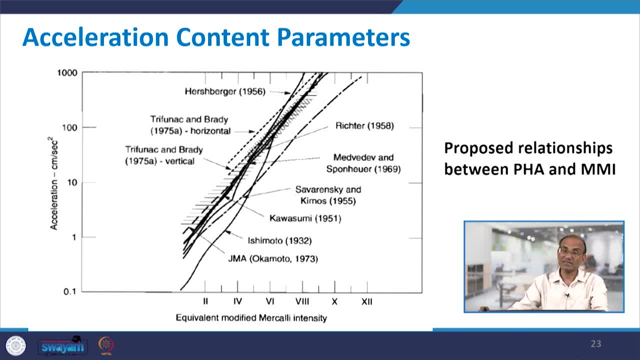 modified Mercalli intensity scale which we have discussed in the last. So there is a relations. So in general you see that the line is going from down to up. that means when, in general, relationships looks linear. Okay, So that means when you increase acceleration value on y-axis, then intensity is going to. 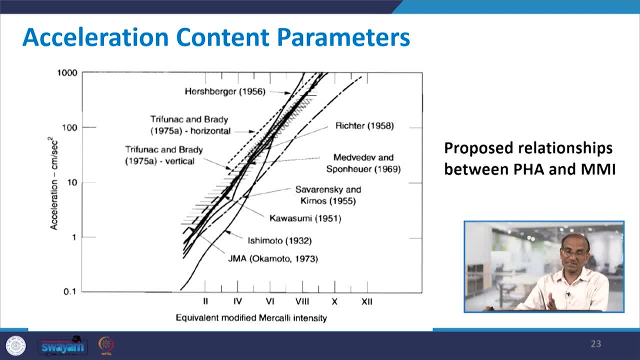 increase, or the other way, on x-axis, when intensity increases, that will require the higher value of acceleration. So kind the linear is kind of relationship is kind of linear. however, different researchers have given different lines but ultimately they fall in a narrow band and you could see. 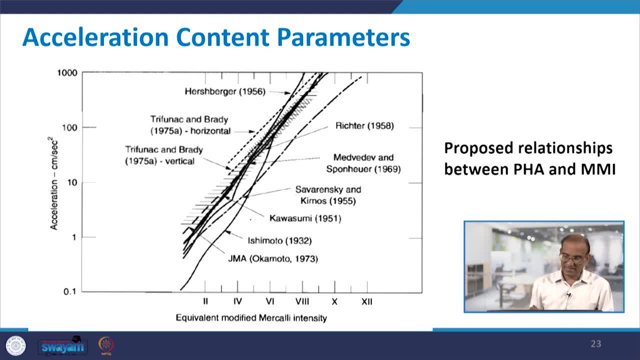 in general, we can say that when this, like acceleration, exceed 100.. Okay, Okay, When this acceleration exceed 100 centimeter per second square, which is roughly 0.1 g, then intensities you get is around 8th. So here you have second, fourth, sixth, eighth, ninth, and then in between you have 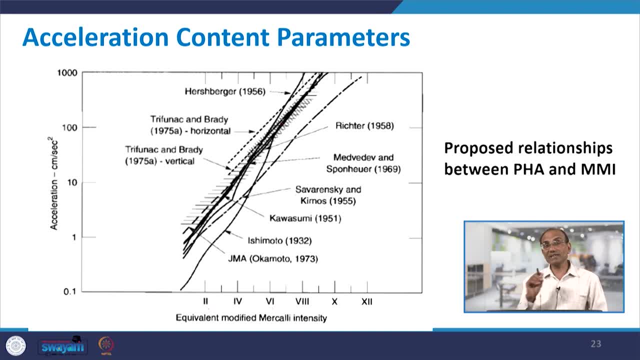 So one thing you notice in the graph: you have linear scale on the x-axis, while y-axis you have the logarithmic scale. So while using this charts, so using this chart, we can roughly get an idea that for given value of, Let us say, acceleration, how much is the intensity? 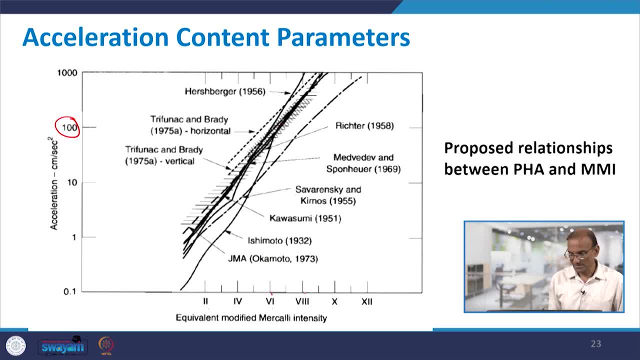 So if I draw, and then here around 6th and 7th, 8th, so you can have this one. So, and intensity is, as usually, represented in terms of Roman numbers, So there should not be a fraction. So if you get the less intensity, suppose I get some value between 6 and 7. then I will. 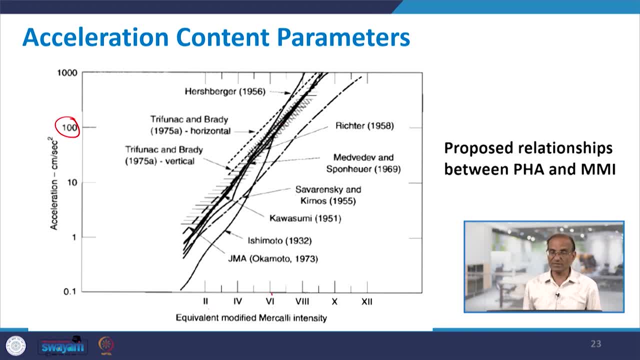 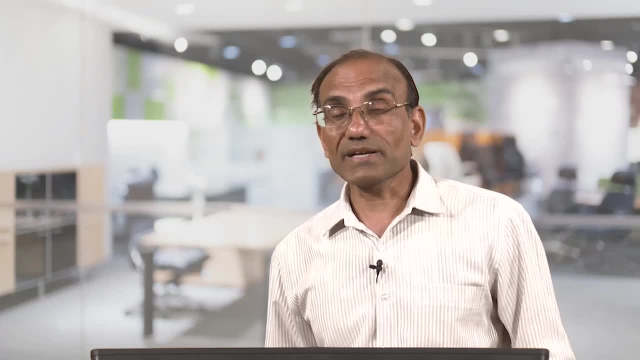 go on the higher side rather than average or, like you know that this in Roman number this should be whole number for intensity. It cannot be 6.5 or 6.8.. Now, coming to the next parameter for characterization of amplitude is velocity. 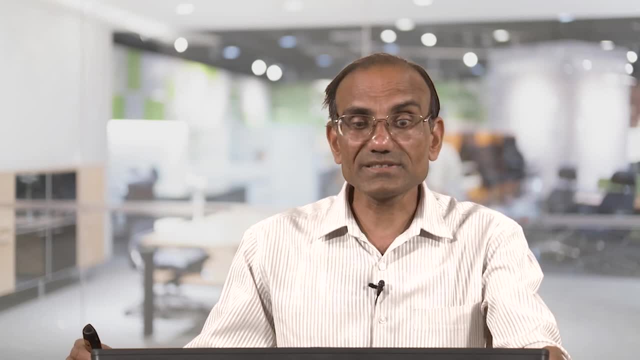 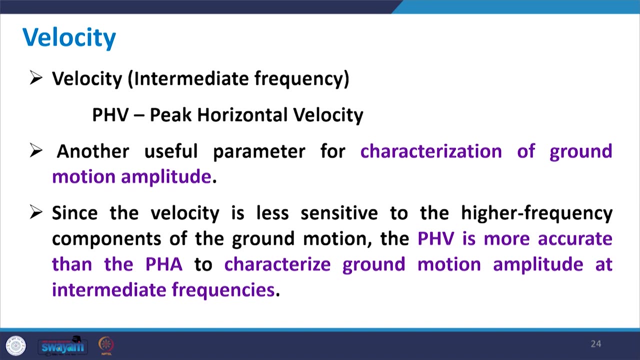 We have discussed lot about acceleration. When we talk about velocity, velocity is for the intermediate frequencies, acceleration is for high frequency, displacement is low frequency, but velocity works at intermediate frequency. and velocity are characterized by the parameter which we call PHV, And PHV is here nothing but peak horizontal velocity. 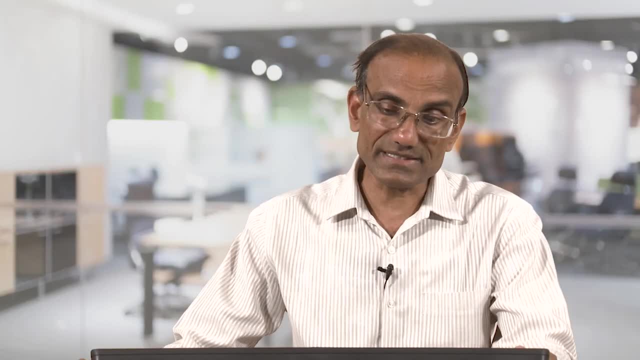 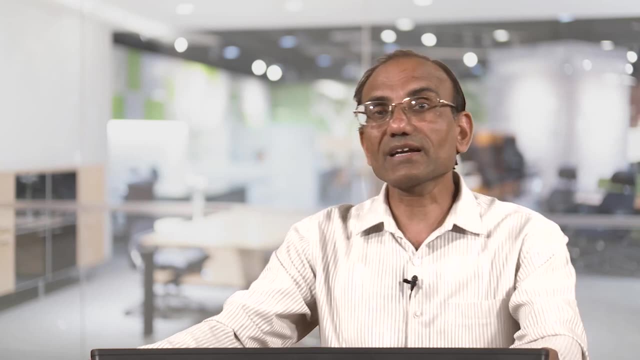 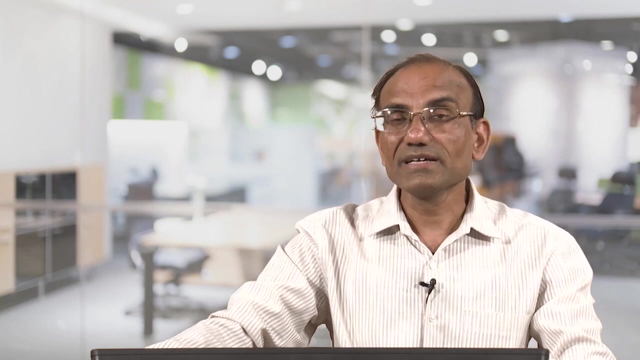 So earlier we have PHA, which was peak horizontal acceleration. Here we have peak horizontal velocity And this is another useful parameter for characterization of ground motion amplitude. Since the velocity is less sensitive to the highest frequency component of the ground motion, the PHV is more accurate than the PHA to characterize ground motion amplitude at. 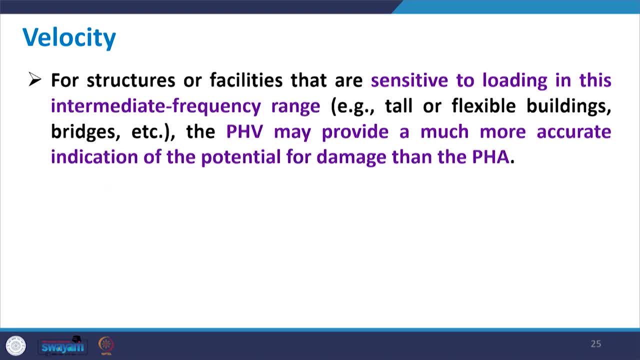 intermediate frequency And this is for intermediate frequency Velocity, for structures or facilities there are sensitive to loading in this intermediate frequencies. for example, you have tall or flexible buildings, bridges, then PHA may provide a much more accurate indication of the damage than the PHA. 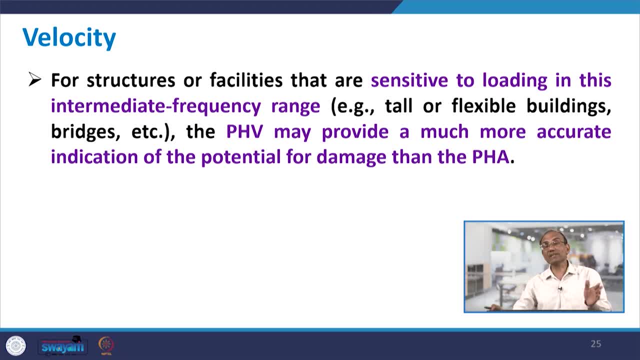 So PHV, that is, peak horizontal velocity, will give you better result than the peak horizontal acceleration, And the reason being because it work in the intermediate frequency range rather than the high frequency range. This work in the high frequency range- PHA for the high frequency, as we discussed. 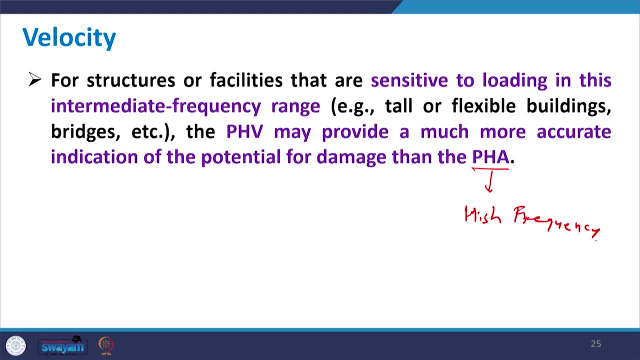 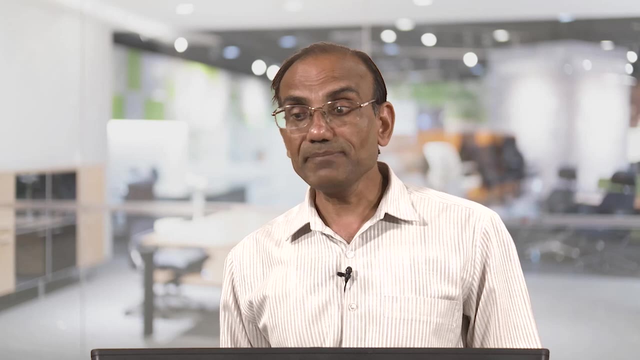 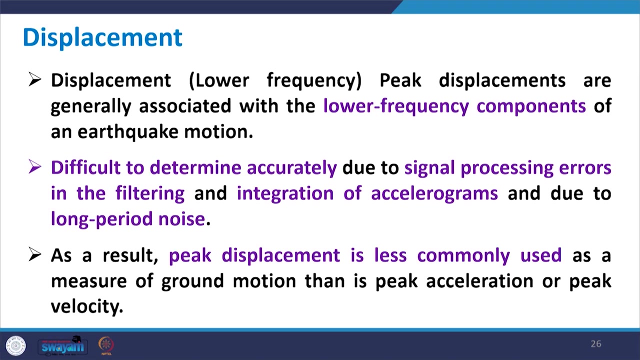 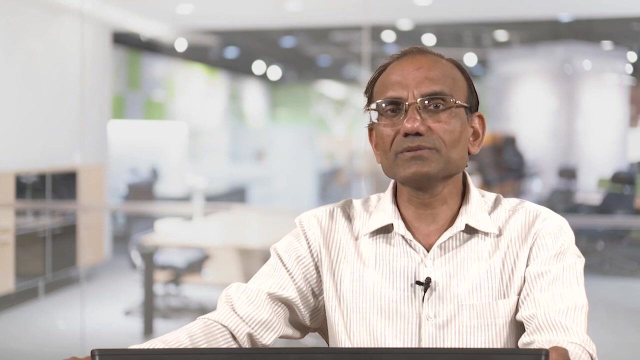 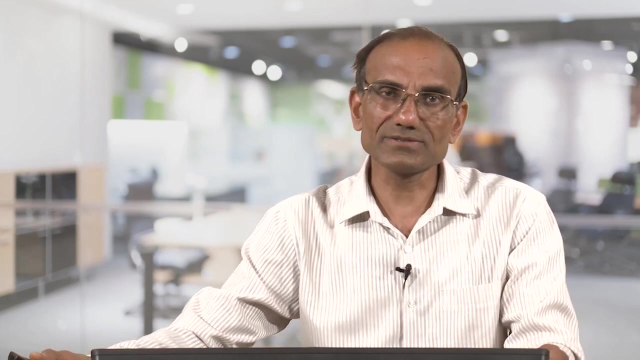 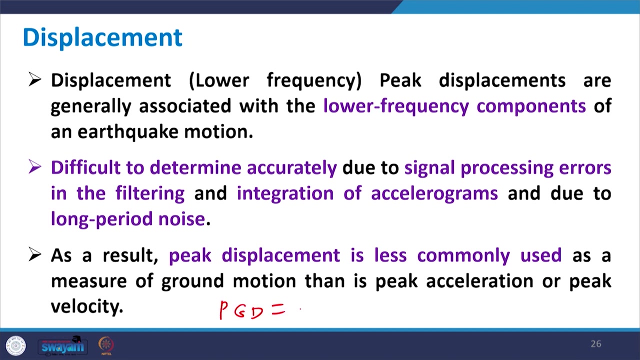 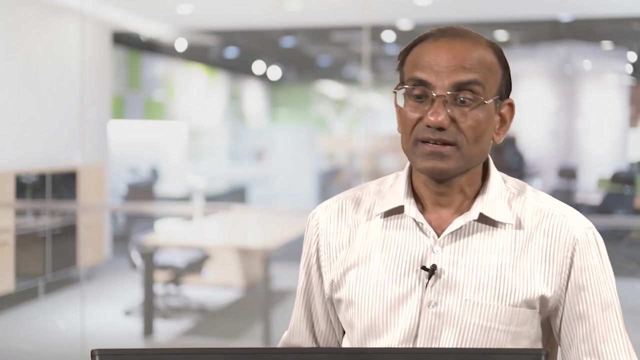 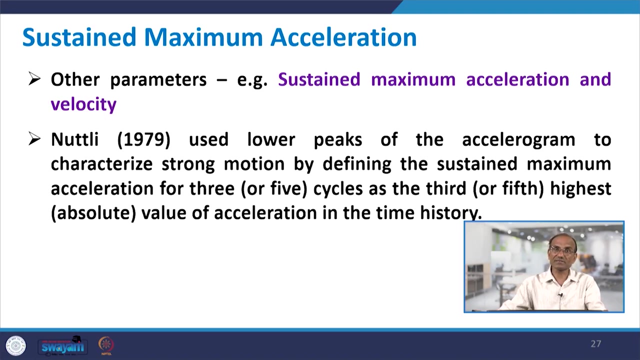 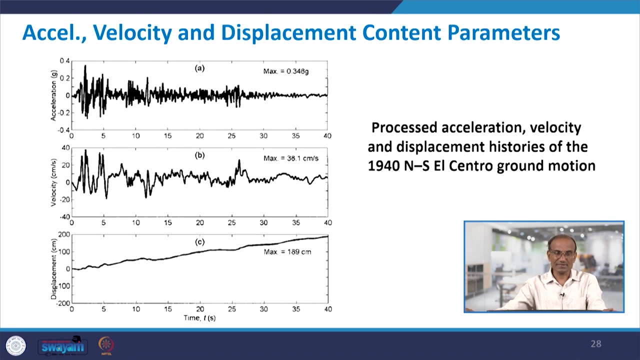 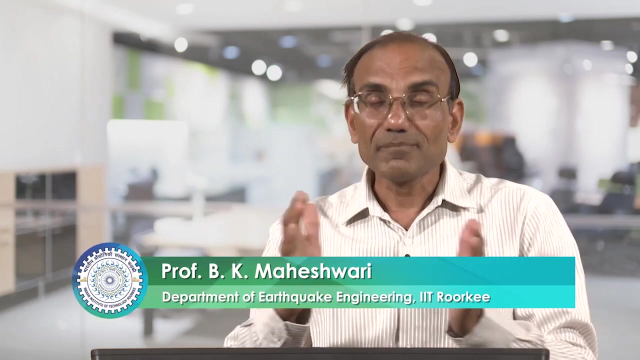 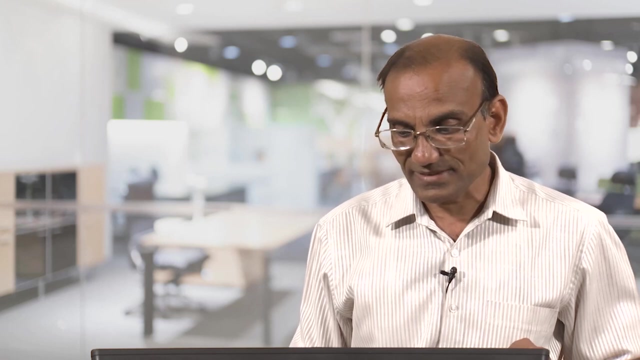 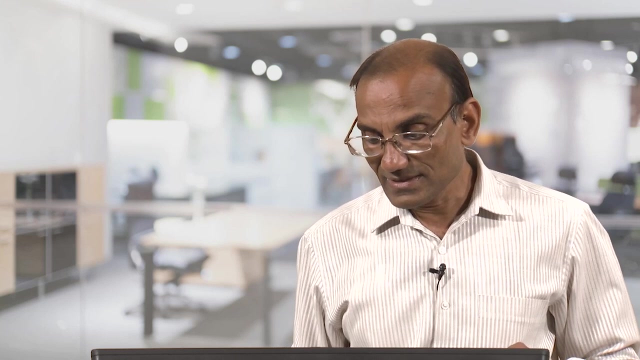 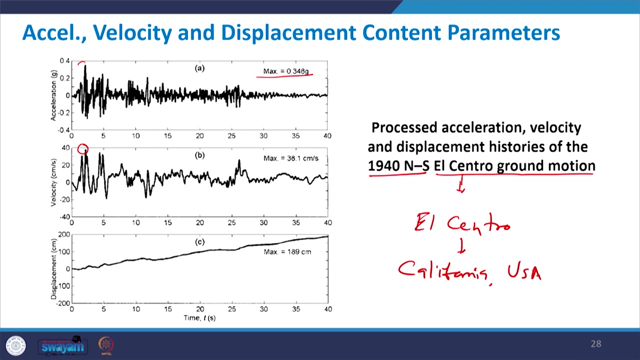 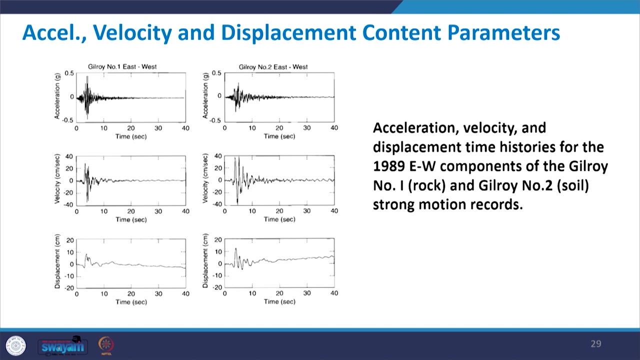 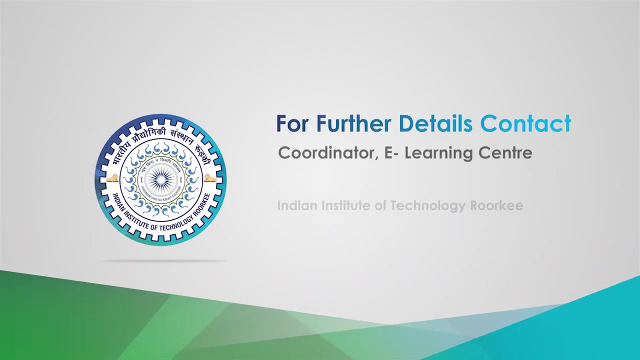 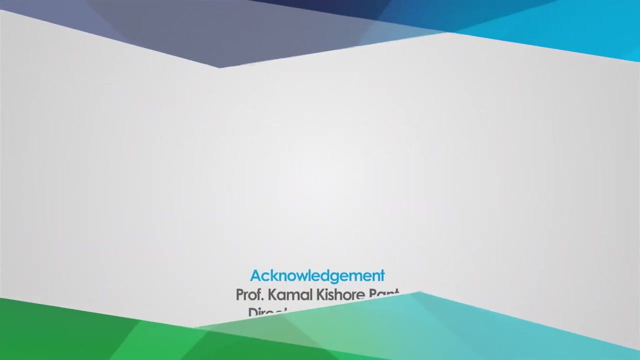 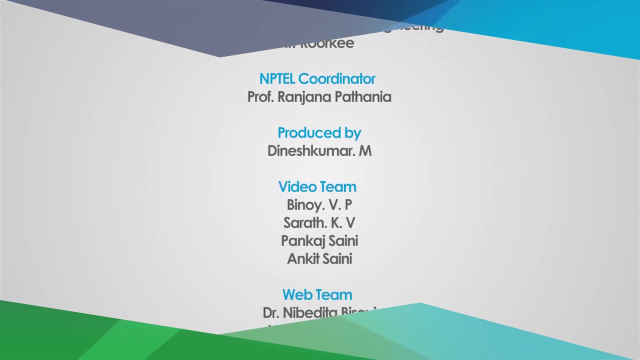 While this PHV, this will work: intermediate frequency, intermediate, Third component. Thank you very much for your kind attention. you.